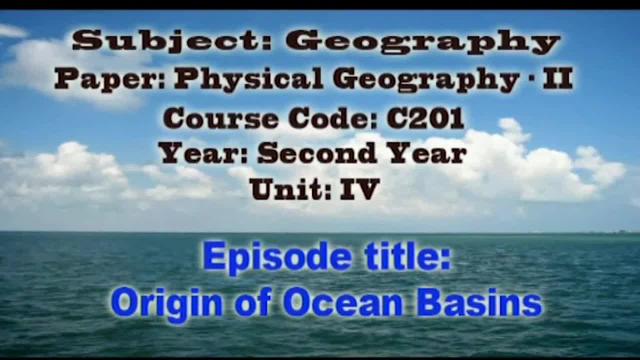 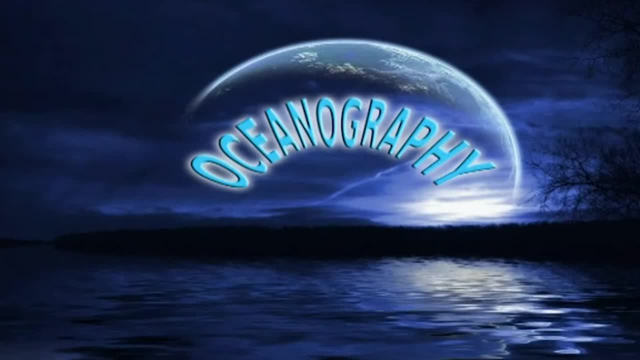 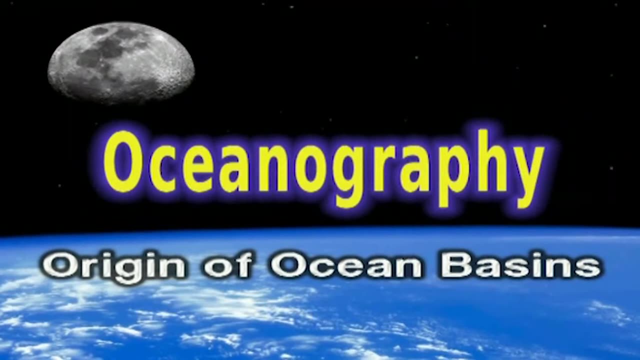 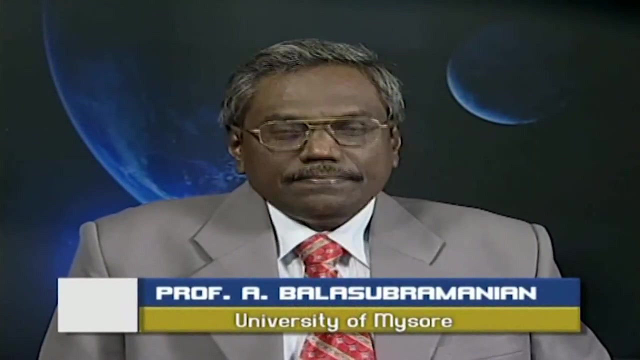 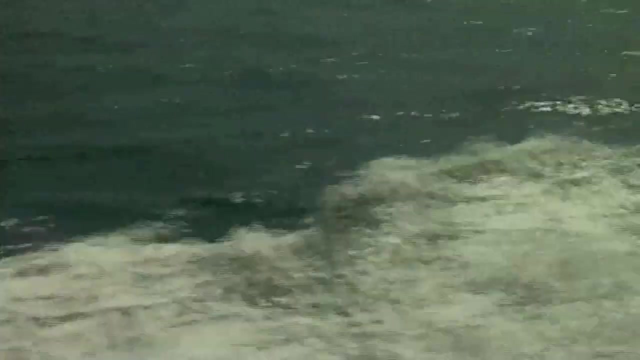 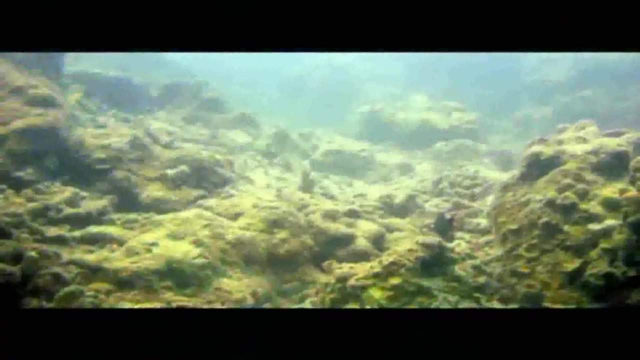 Namaskar. The topic of discussion today is on origin of ocean basins. Oceanography is the scientific study of seas and oceans. It is an interesting and interdisciplinary science. It includes the subjects like geography, geology, chemistry, physics, biology, climatology and. 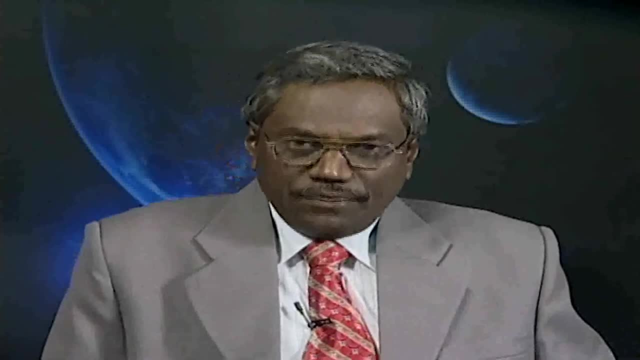 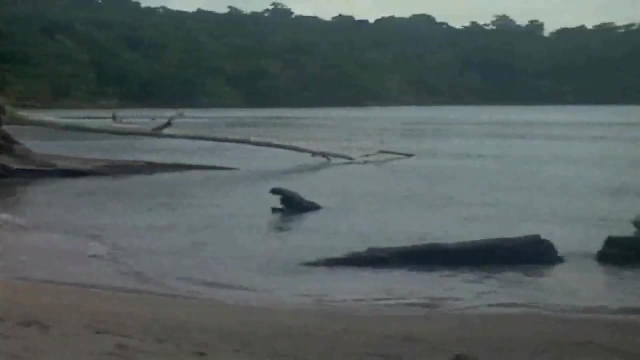 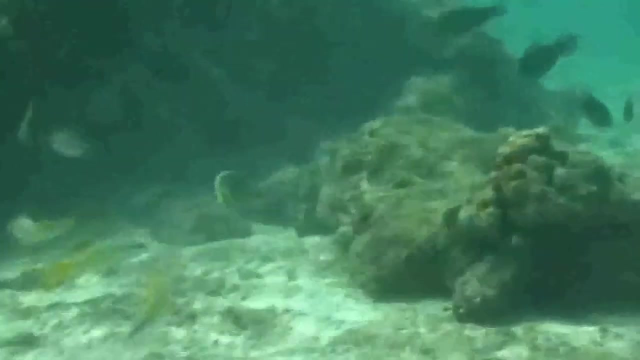 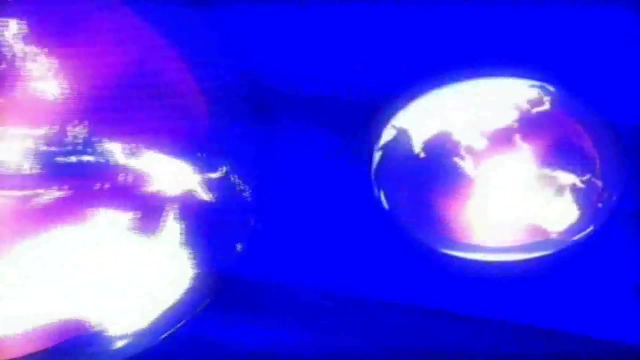 engineering. Oceanography mainly deals with the following aspects: The geological features of ocean bottom. physical conditions with reference to ocean water and its temperature. chemical composition of sea water and marine sediments. biological conditions of marine life, which include the fauna and flora. the role of oceans in controlling the global climate. 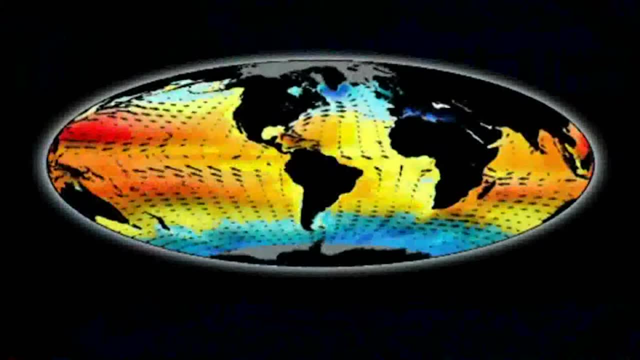 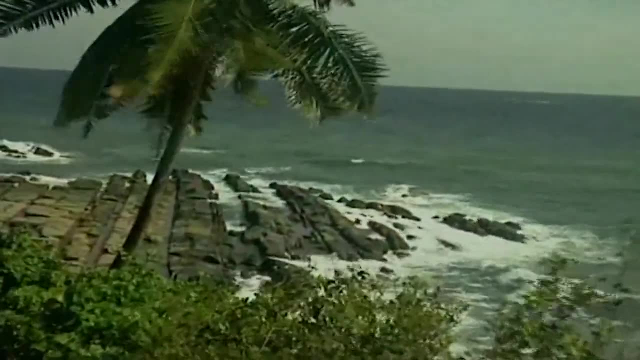 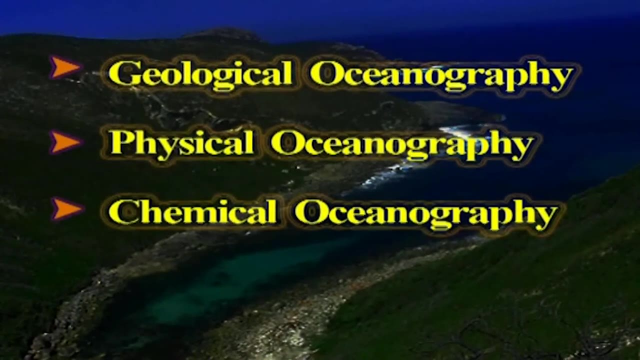 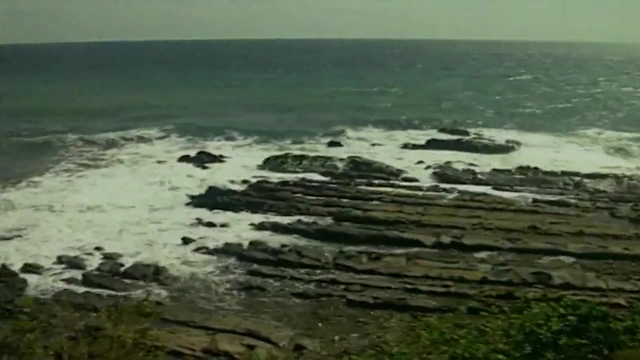 navigation and the economy. The origin of ocean basins is an important aspect in oceanography. Oceanography is also further divided into geological oceanography, physical oceanography, chemical oceanography. The geological oceanography deals with several aspects of seas and oceans. The essential 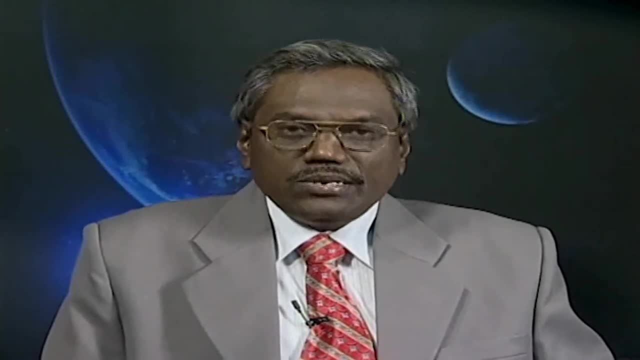 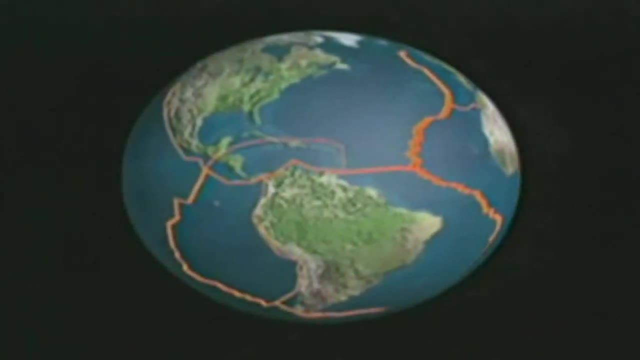 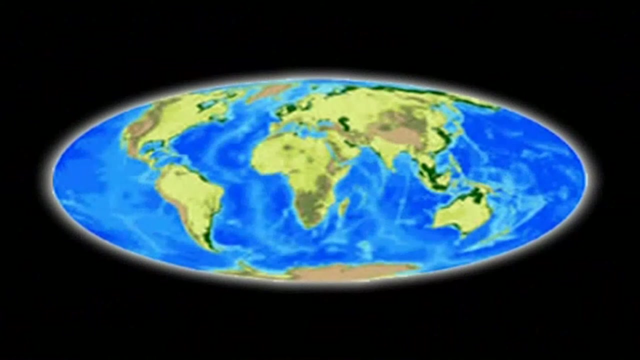 aspects are: origin of water and air on the earth, theory of continental drift and crustal blocks, theory of plate tectonics and continuing dynamics of ocean basins, the spreading of sea floor, the distribution of ocean basins and coastal geomorphology. 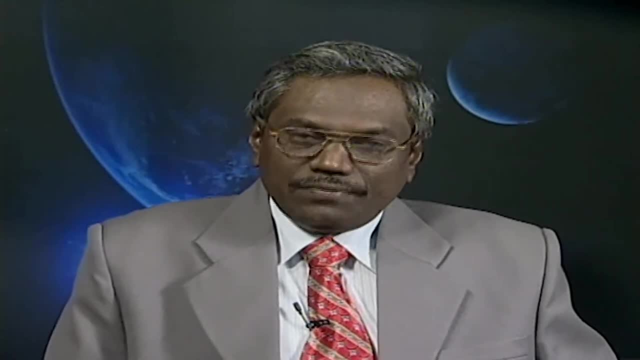 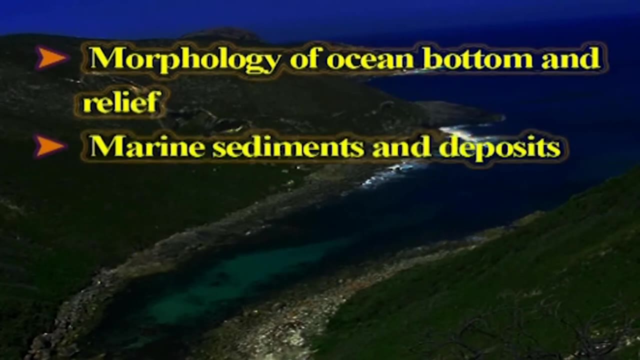 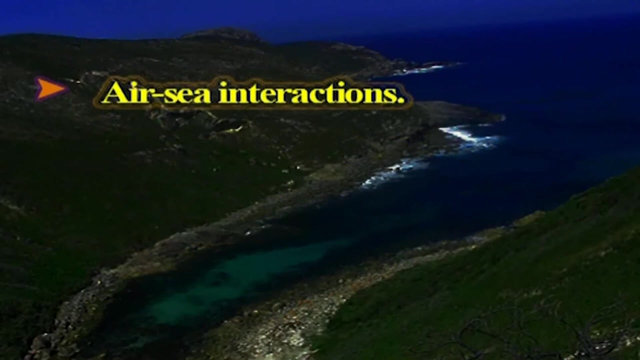 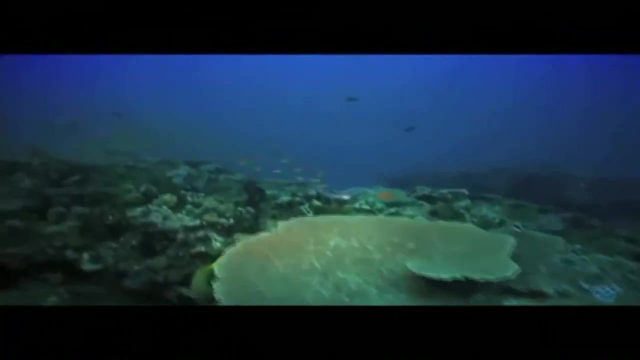 The geological oceanographic studies also deal with the following aspects: Morphology of ocean bottom and relief, marine sediments and deposits, coral reefs and beach processes, coastal disasters and management, air-sea interactions and the study of marine sediments, submarine canyons, underwater topography and corals. At present, earth has about 1.3 billion cubic meters of ocean surface. The geological oceanographic studies also deal with the following aspects: Morphology of ocean bottom and relief, marine sediments and deposits, coral reefs and beach processes, coastal disasters and management. 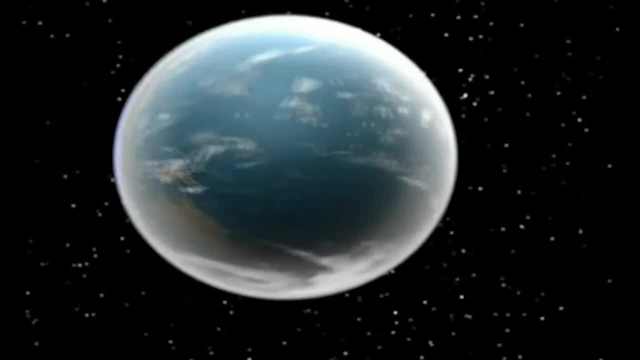 air-sea interactions and the study of marine sediments, submarine canyons, underwater topography and corals. At present, earth has about 1.3 billion cubic meters of ocean, The geological oceanography kilometer of water. This amount is present mostly in the form of seas and oceans, Because 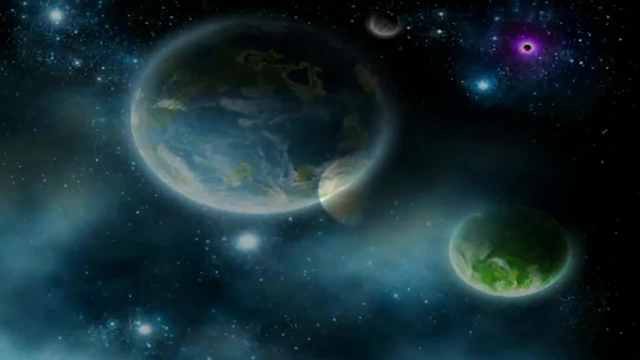 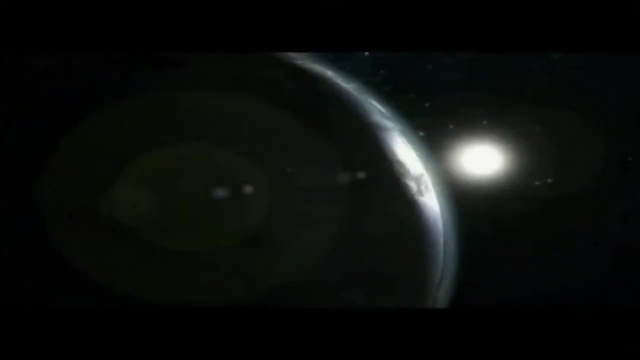 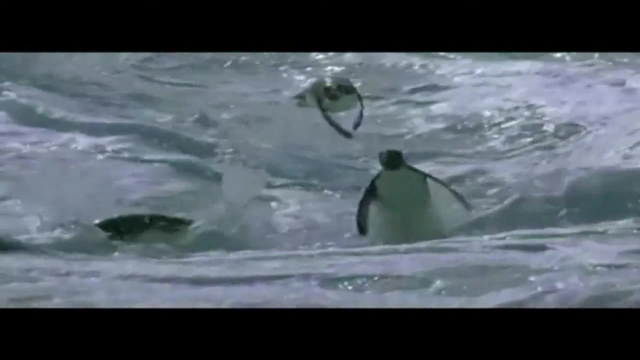 of this, the earth is called as a blue planet. Three important spheres make the planet earth as a unique member of the solar system. They are the atmosphere, hydrosphere and the lithosphere. Their combined role lies in the sphere of all living systems on earth. First of all, 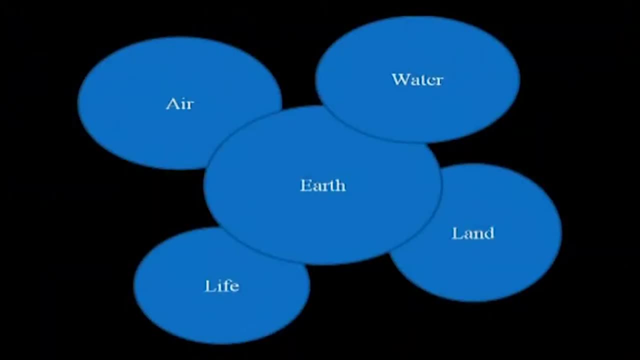 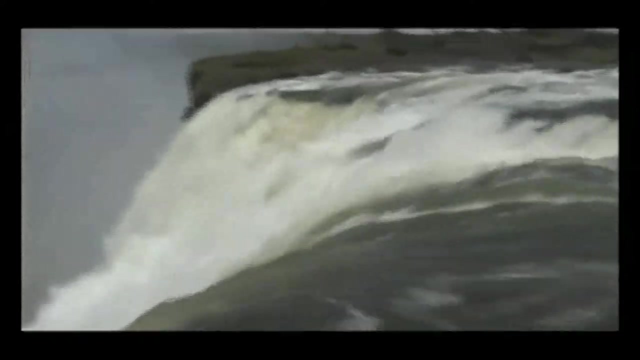 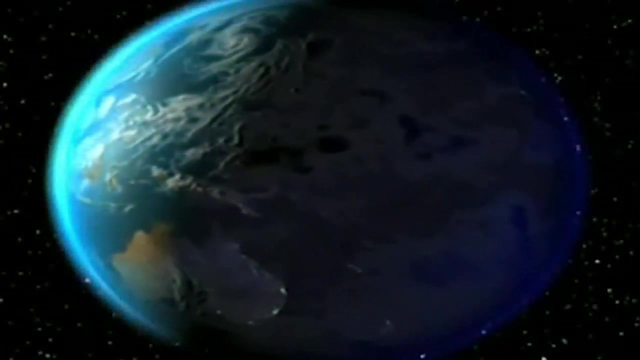 it is necessary to understand the origin of land, air and water on the earth. The origin of water and air on earth is almost related to each other. The reason for the occurrence of such a huge mass of water on the globe is still a myth and reality. The reason goes. 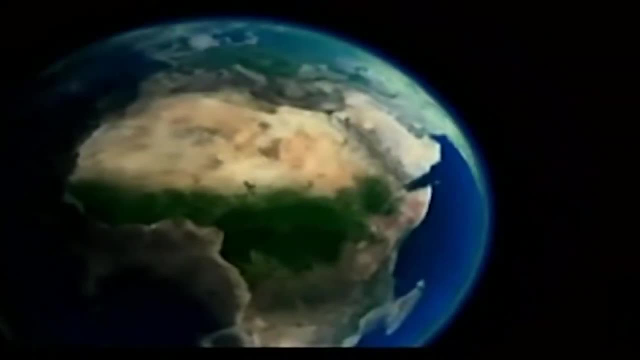 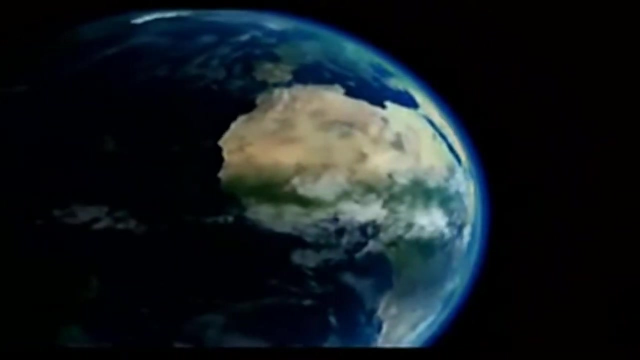 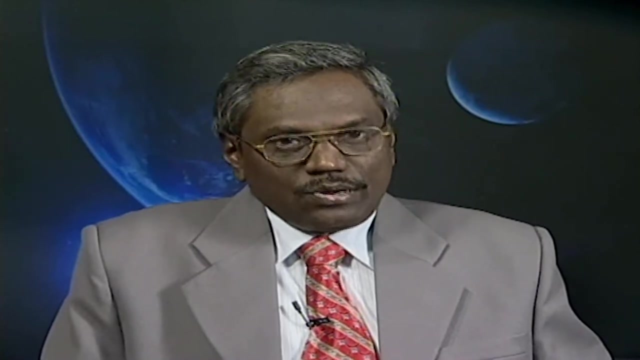 back to the origin of earth itself. The exact mode of origin is not precisely known. even today, Scientists assume both primary and secondary sources of water. The primary sources would have given rise to both air and water on the earth. Two possible sources, as internal source or external source, have been proposed so far. Some of them are: 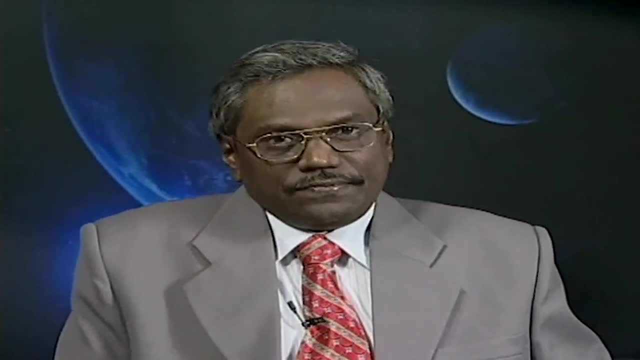 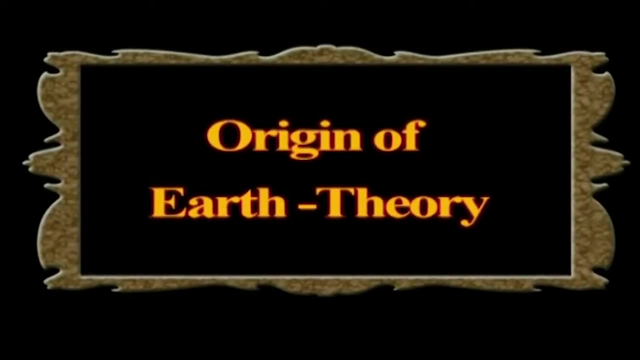 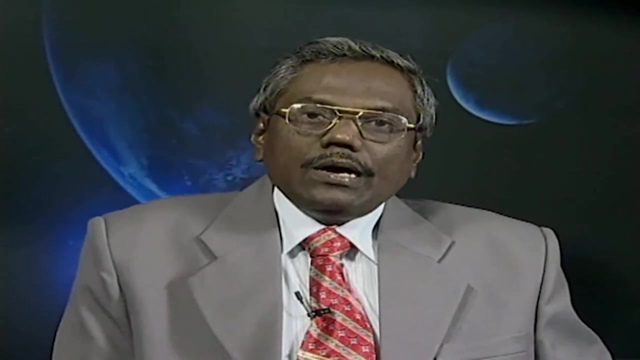 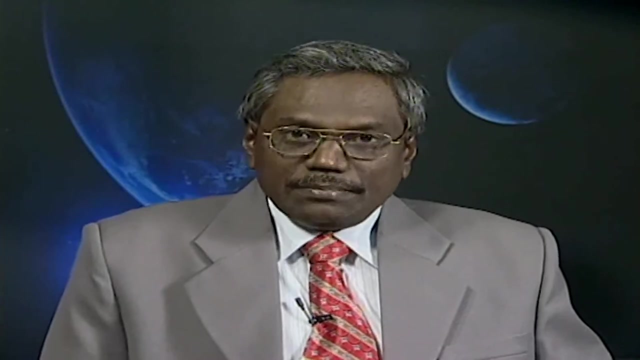 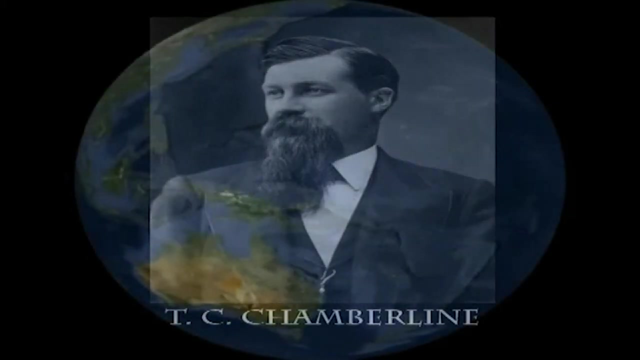 attributed towards the theories of origin of earth itself. Let us see the origin of water. Let us see the origin of water. Many theories have been proposed so far. The planetesimal hypothesis of 1749, proposed by T C Chamberlain on the origin of earth, was probably the first idea about the birth of 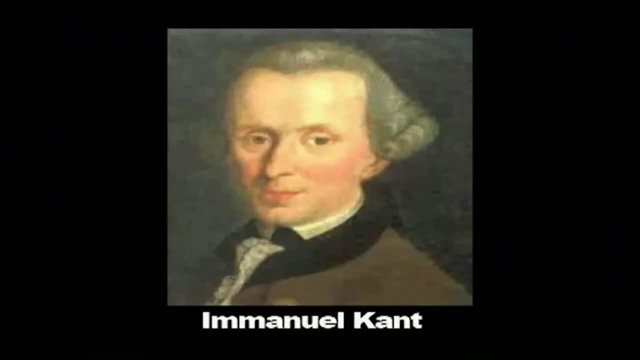 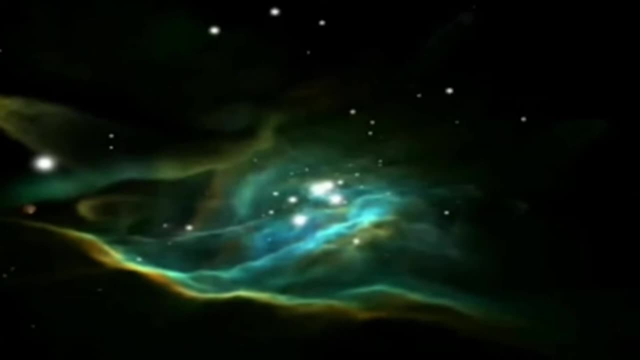 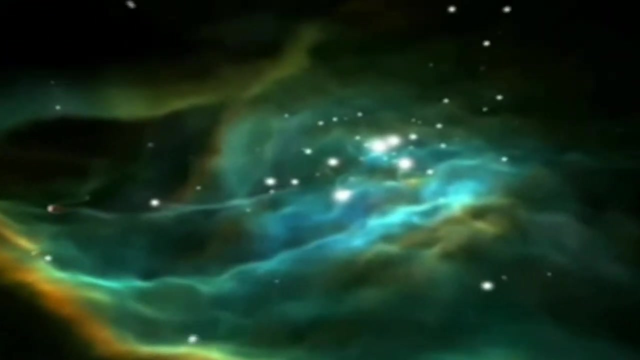 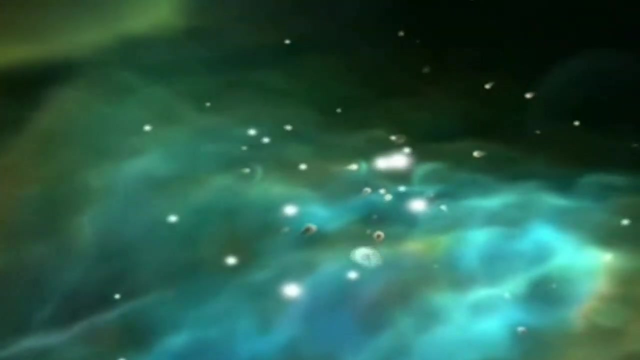 the earth. Later, in 1755, Immanuel Kant has proposed the ancestral nebula theory. Nebula containing cloud of gas and dust leading to the generation of planets from the sanguine reason was the theory proposed by Immanuel Kant. The nebula was considered as a hot gaseous material and hot gaseous nebula was thought. 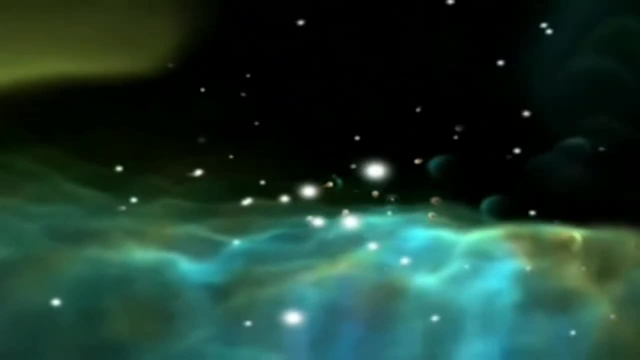 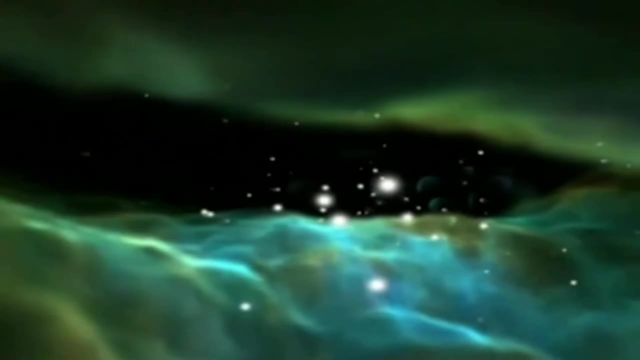 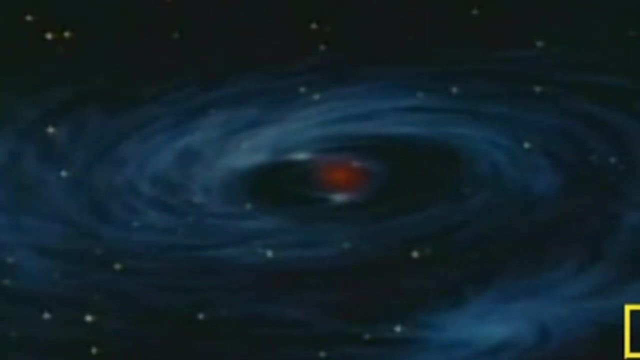 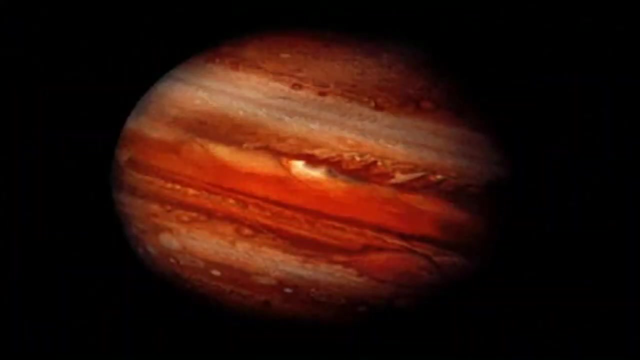 to be rotating with great rapidity. initially, It also underwent cooling and contraction, due to which the speed got increased. Due to strong centrifugal force along the equator, the materials were thrown away as successful rings. These rings cooled down to form solid and liquidous masses. at a later stage, The same process have happened to planets to form. 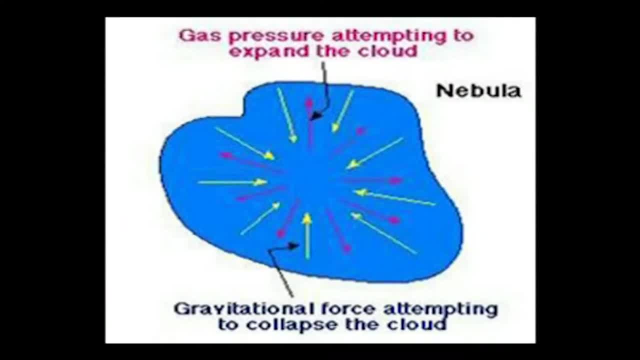 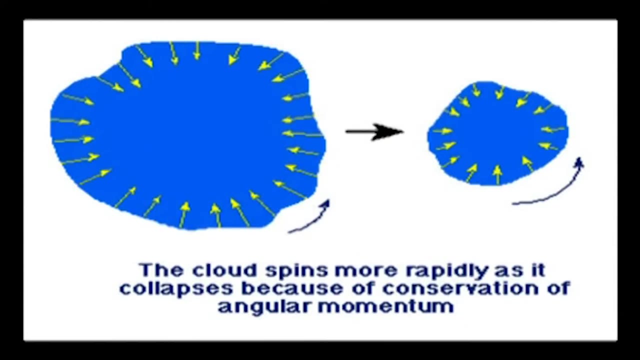 their satellites also at a later time. This diagram shows the structure of a nebula where the gas pressure is attempting to expand the clouds. This diagram shows the equatorial bulge of the nebula, which gradually increases and gradually gets detached from the nebula in the form of rings. 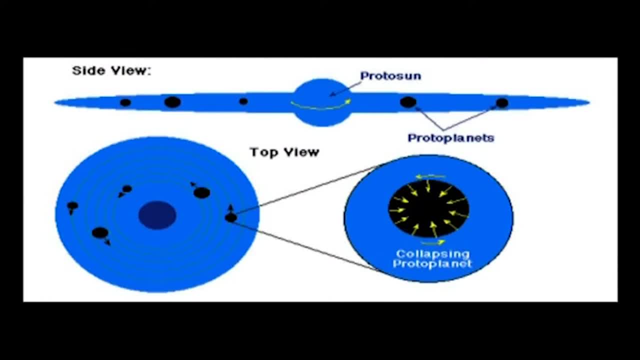 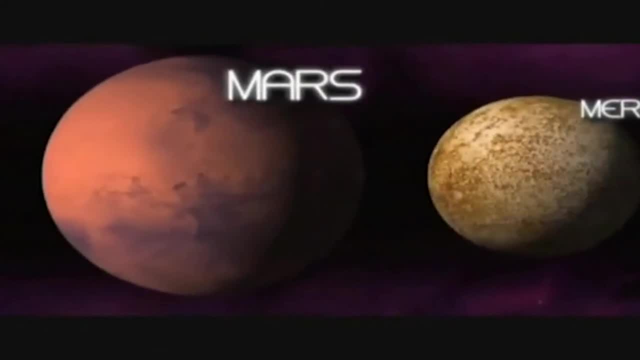 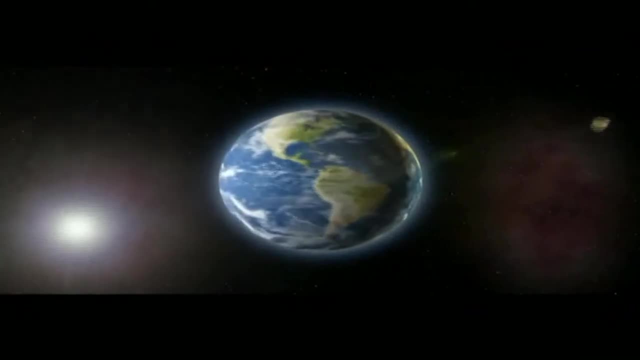 This diagram shows the release of protoplanets, which happened in sequence. Collapsing protoplanets further release their masses as satellites. The ultimate celestial output are the birth of various planets. The first set of protoplanets were released with more gas available with the parental source that might have come as 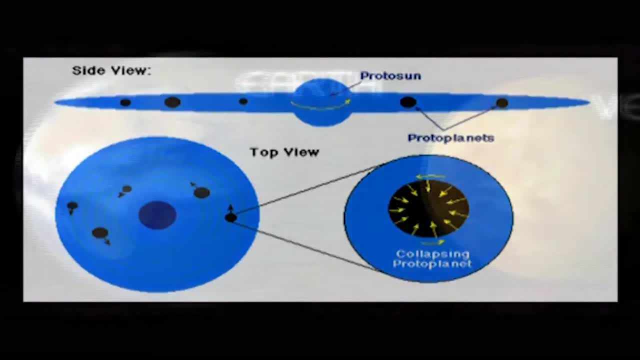 a flat ring. It will also have the upper flow and also some gas flow that may have a more fluid form. These are called nebula-shaped rings planets. one by one, The bigger size of all outer planets came in because of this Outer 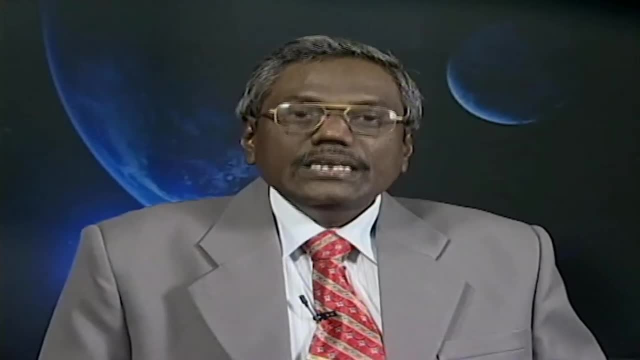 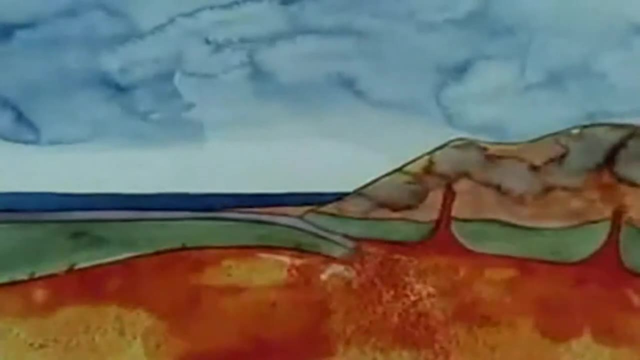 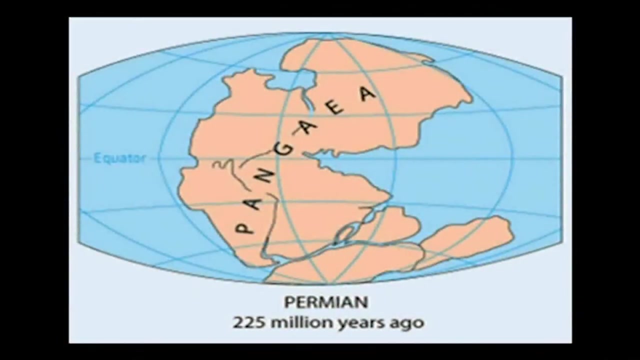 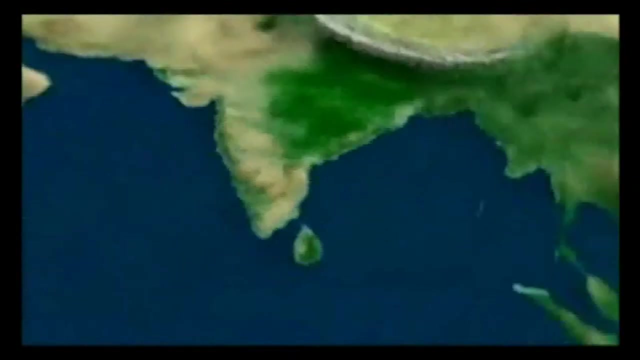 planets are also lighter planets. Initially, embryonic continents were formed due to cooling. Partial melting of the mantle produced the volcanic rocks like basalts that were little in silica. Origin of a single continental mass was created. That continent was called as Pangaea. The name Pangaea means all earth. Pangaea was a supercontinent consisting of 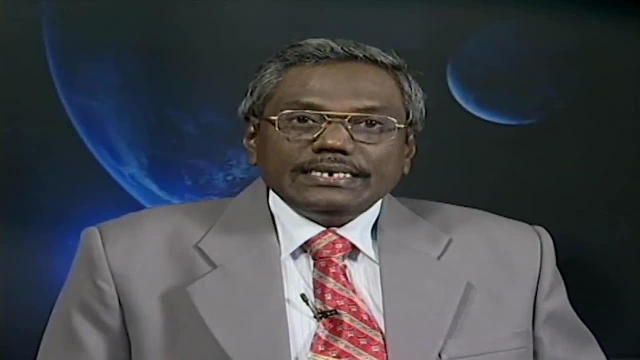 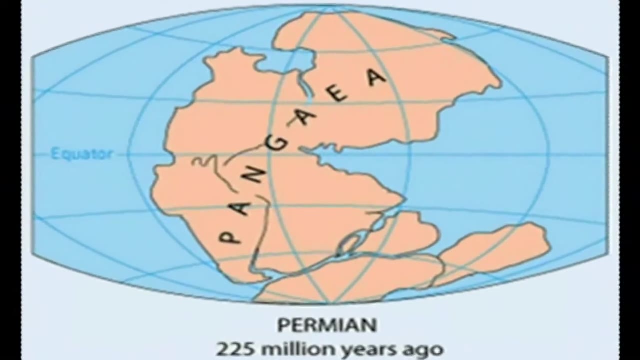 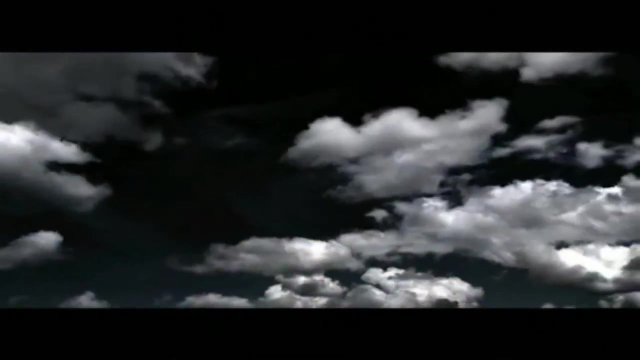 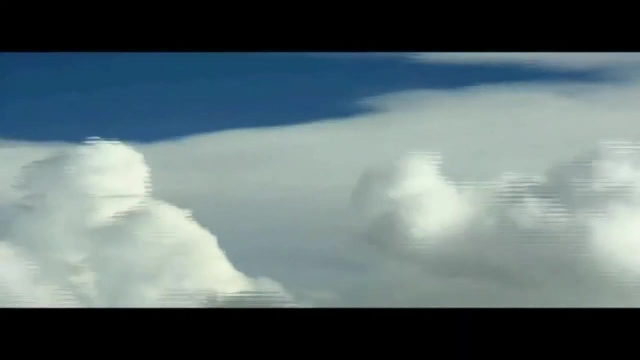 all the earth's landmasses. It existed from the Permian period through Jurassic period. This diagram shows the structure of Pangaea, roughly about 30 years old. Outgassing from the earth's interior has poured out water masses through eruption and other reactions with the atmospheric gases. Atmosphere also helped with sufficient pressure. 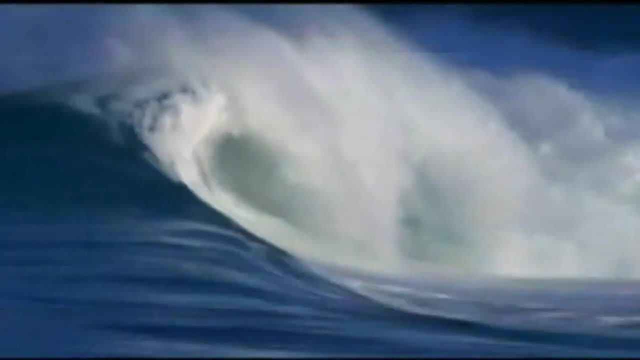 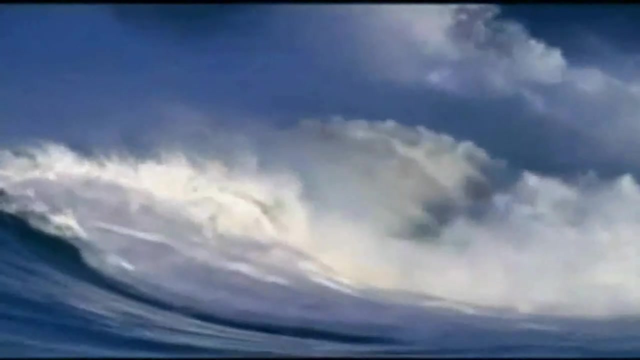 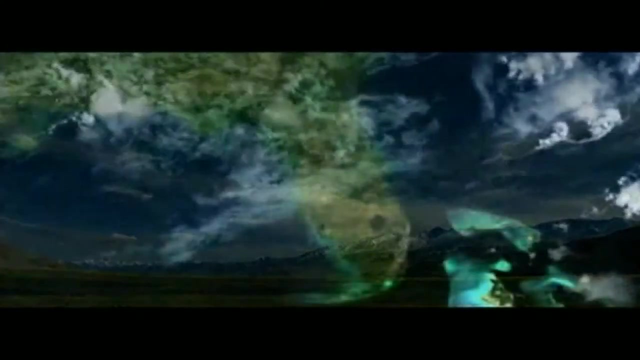 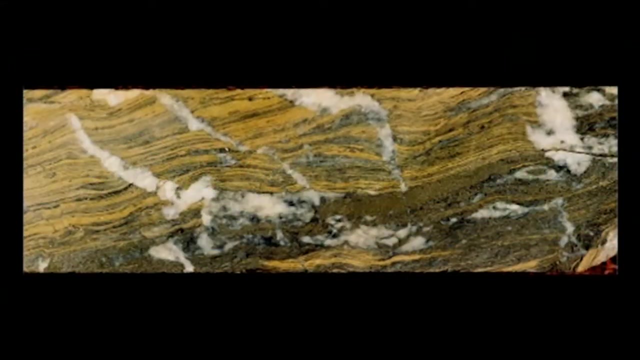 for precipitating the water on the planet. Condensation and precipitation continued for several thousand years to form the oceanic water masses. Infant earth grew in size and successfully in capturing free atmospheric molecules to form water masses. People also attributed to the biochemical synthesis through mineralization and photosynthesis for the 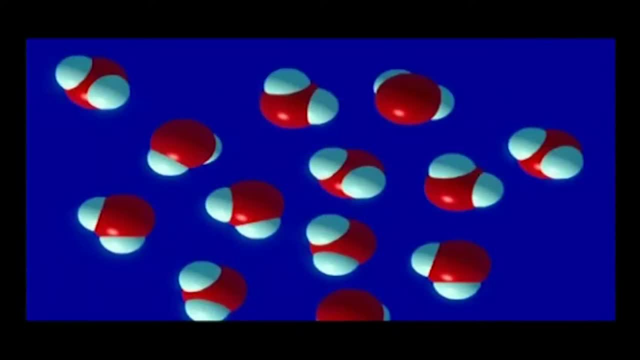 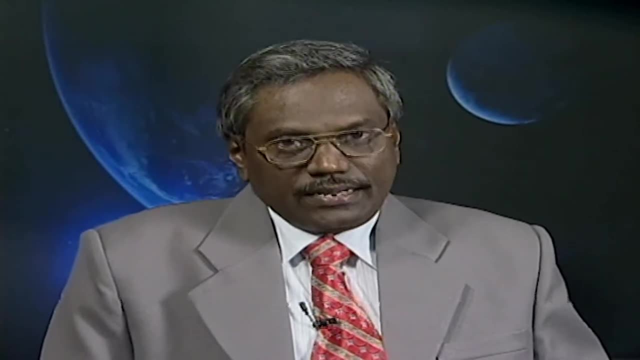 presence of water on the earth. Radial leakage of water molecules stored in hydrous minerals of the earth's rocks was also considered as a contributing factor for water on the earth. Photolysis � device was also another mechanism. The nematode like formation of water molecules 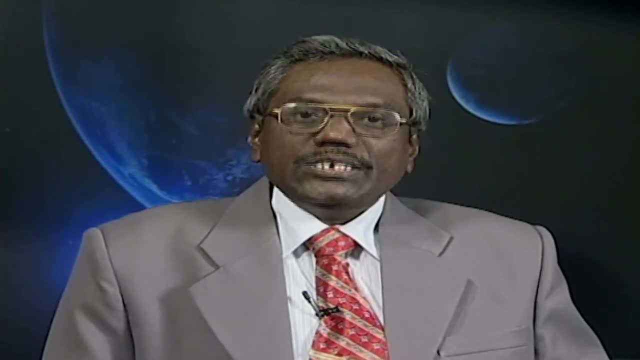 in water is similar to that of the meteorite, but a moment I can say that the night is not unsatkable Under water analysis ofément. these are all the results ofGI Thermovernicle's. The radiation can break down chemical bonds on the surface of chemical masses. The next category belongs to the internal sources. A sizeable quantity of water would have been available within the material which formed the earth initially. Water molecules would have escaped earth's gravity more easily when it was less massive during its early stage of formation. The internal sources provided carbon dioxide, water vapour, nitrogen. 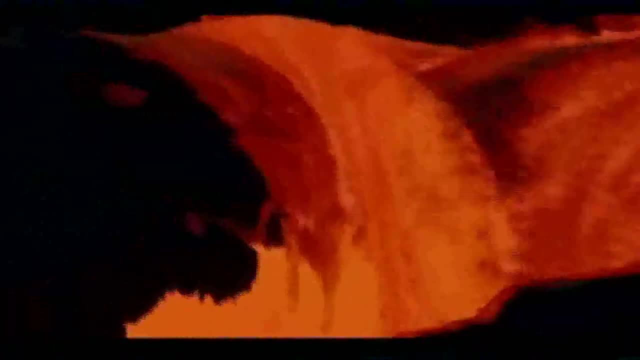 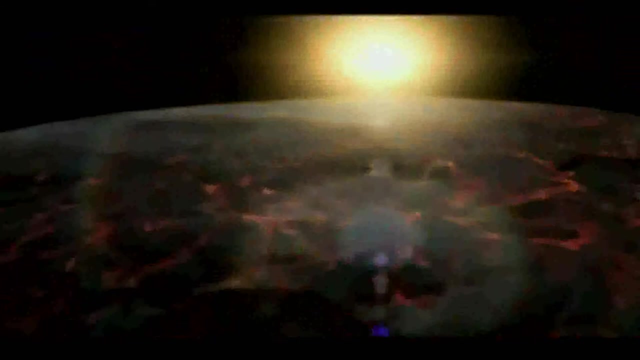 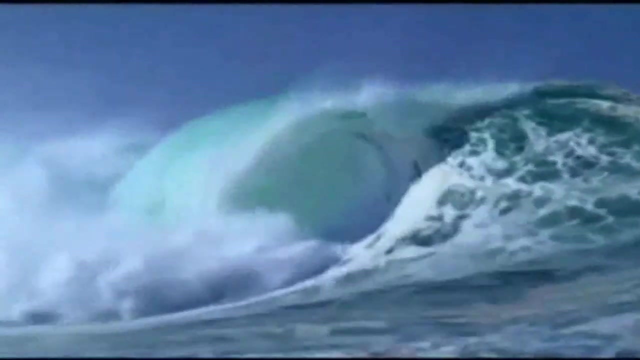 and other gases also. Many gases were provided by volcanic eruptions, hot springs and geysers. All of them are earth-born sources. Primitive oceans were first formed from the water molecules released from the interior and also the atmospheric precipitation. These water bodies joined together. 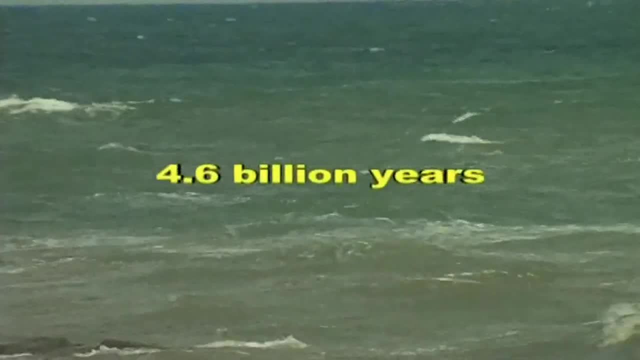 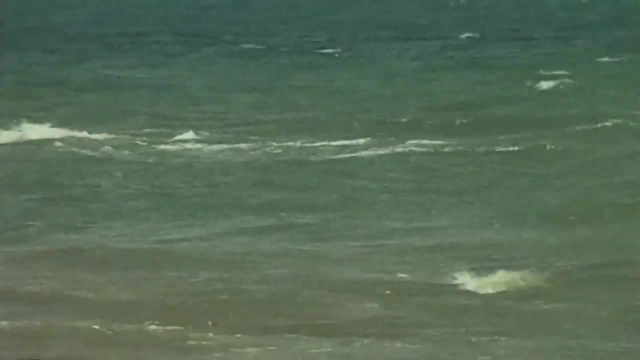 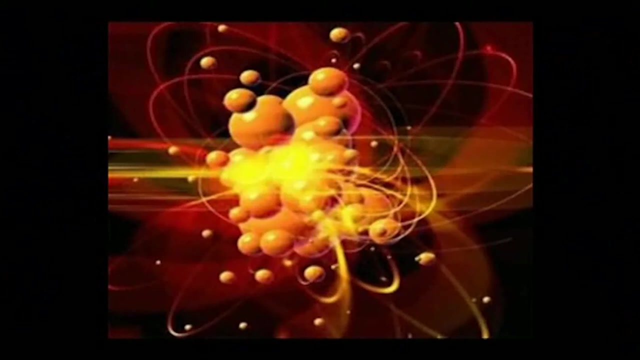 to form seasoned, interconnected oceans over a period of 4.6 billion years. The extra-terrestrial sources also thought of contributing for water on earth. People also attributed that the earth's water was originated purely from comets. This was done as a result of measurements. 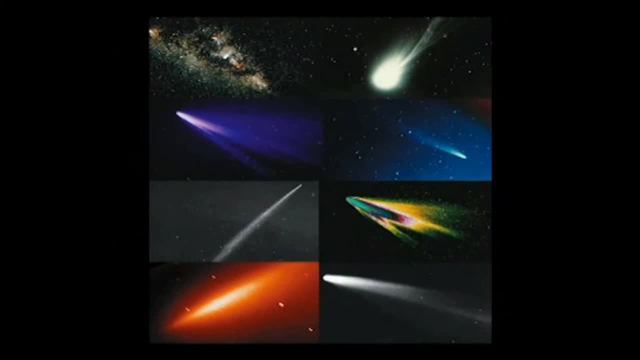 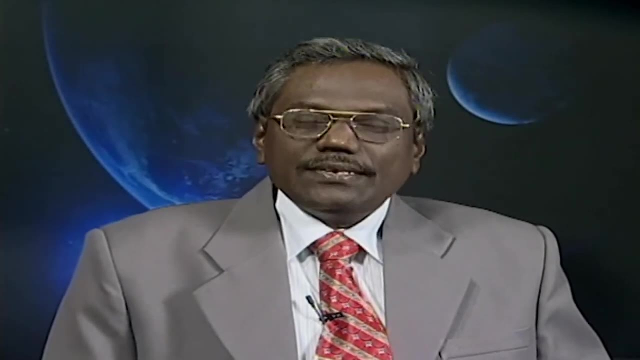 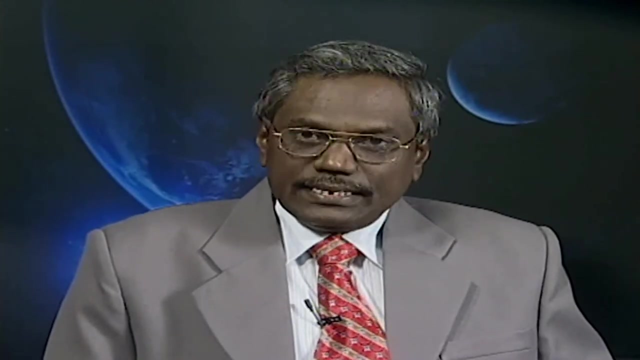 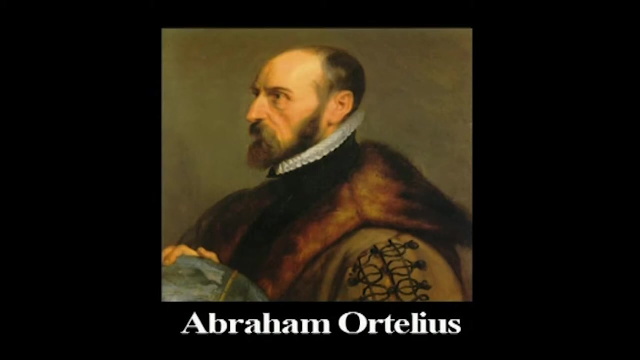 of the isotope ratios of hydrogen in the three comets like Halley, Heoctek and Haleepopp. The shapes of continents on opposite sides of the Atlantic Ocean was noticed by several scholars. Even today we amazingly see this feature. It was in 1596, Abraham Artelius put forward the hypothesis of continental drift In 1858. Antonio Snyder wrote a entry into the humanities of mathematics. I am proud to say that some of these keywords are still being used today. It is important to note that the continental drift as a dimension of the ocean is the difference between the continental drift and the drop-srub of the water. I am confident that we have found a solution for this model. I hope you found this solution and can help us realize the potential for the future. I hope you like this information. I would like to thank mycom. 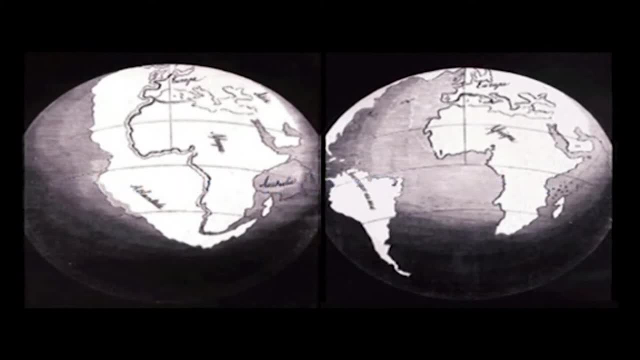 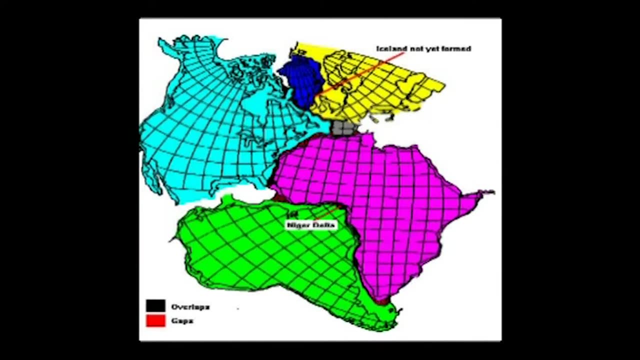 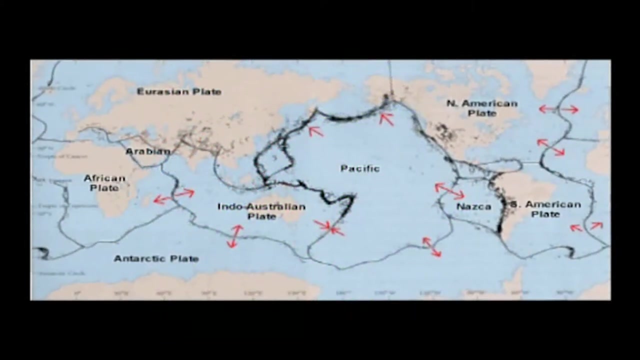 Pellegrini illustrated the closed and opened Atlantic Ocean with a diagram. This is the diagram which has been proposed by him. One can see all these features in this illustration: that many of the continents are united together, with their boundaries similar to each other. 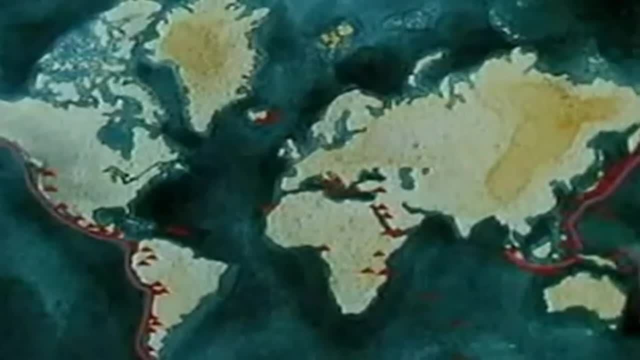 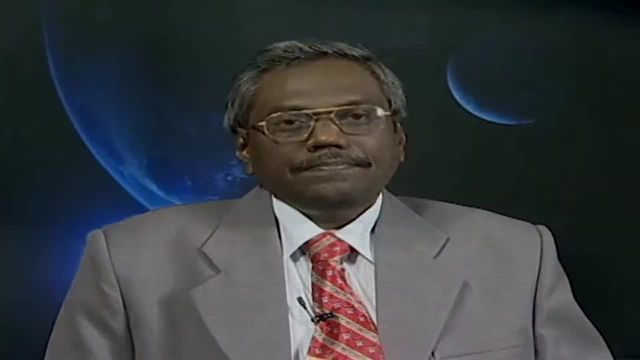 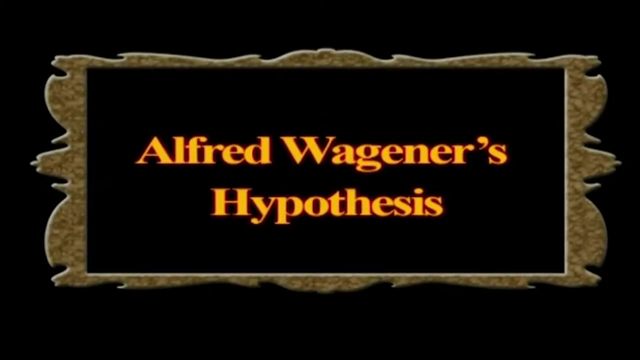 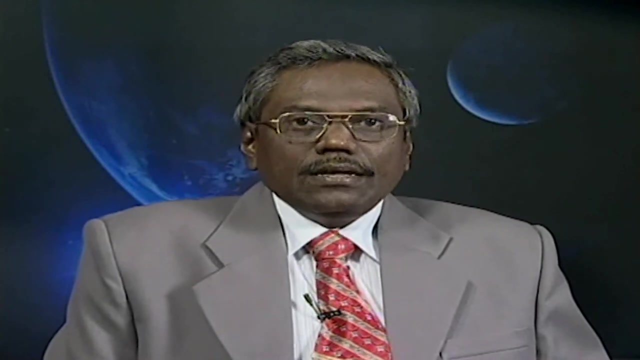 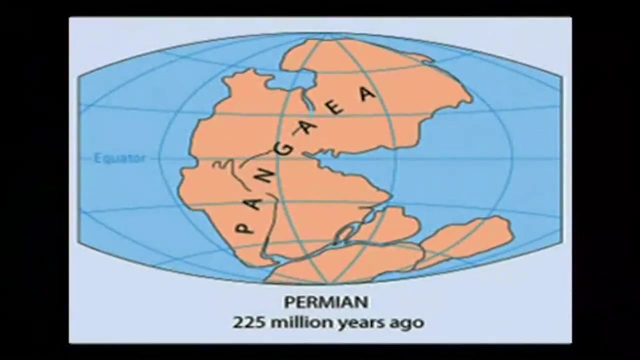 These observations forced the ancient scholars to work on the distribution of continents. This led the birth of continental drift theories. initially, Let us see the Alfred Wegener's hypothesis. According to this concept, about 200 to 300 million years ago, all continents were attached together as a single landmass. That single 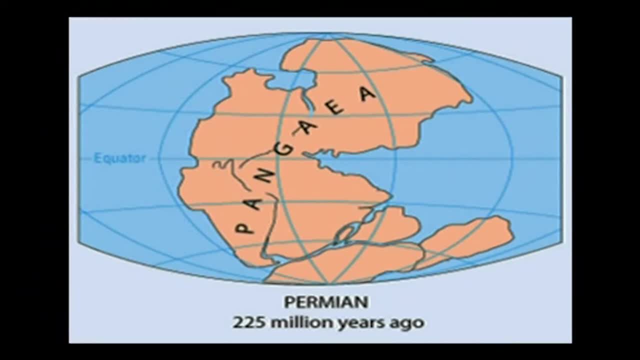 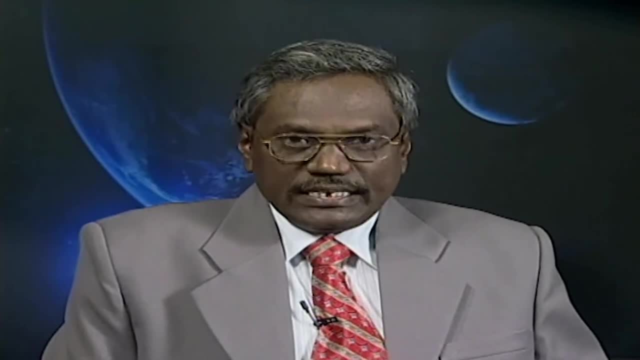 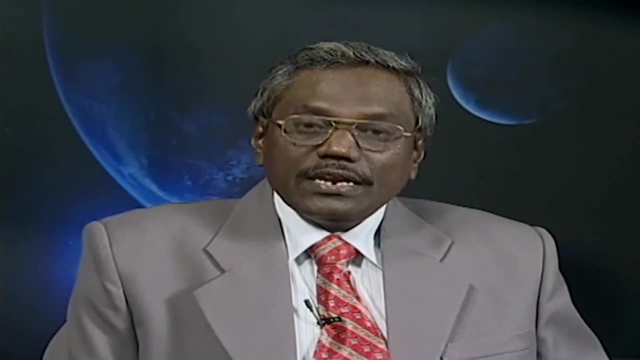 landmass was called as the Atlantic Ocean. The knoll was designed as the super continent Pangea. Thermal expansion and volcanic activities broke the Pangea into new continents. These new continents drifted away from each other due to further expansion of rip zones. Wegener was the first to use the term continental. 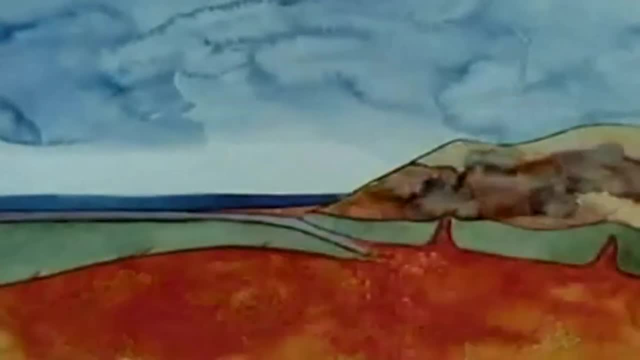 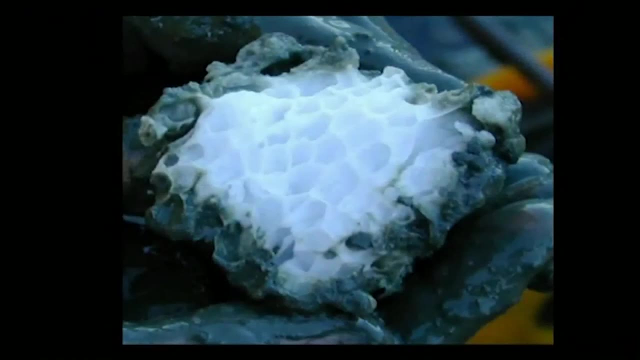 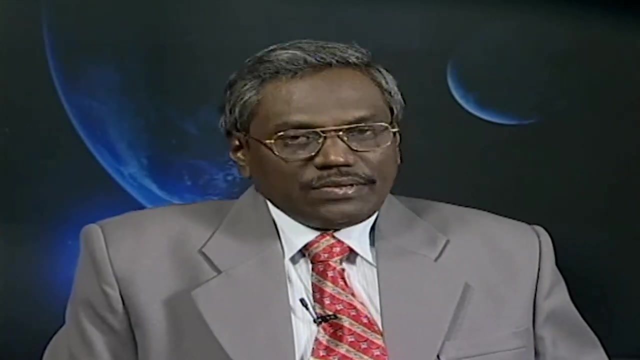 drift. There are several evidences available on earth to support the theory of continental drift. Similar fossil patterns appear on earth. The large structure of the earth is known as the evidence across many adjacent countries is one among them. The Mesosaurus skeleton freshwater reptile found in Brazil and South Africa is another. 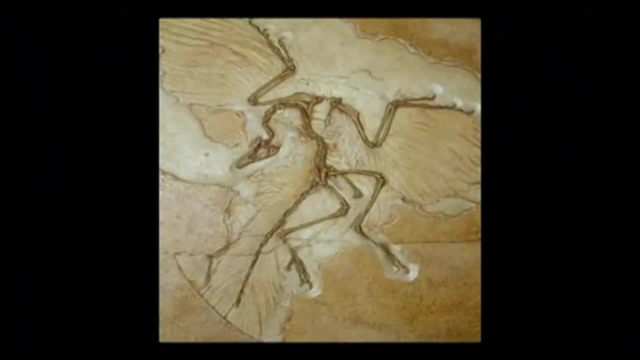 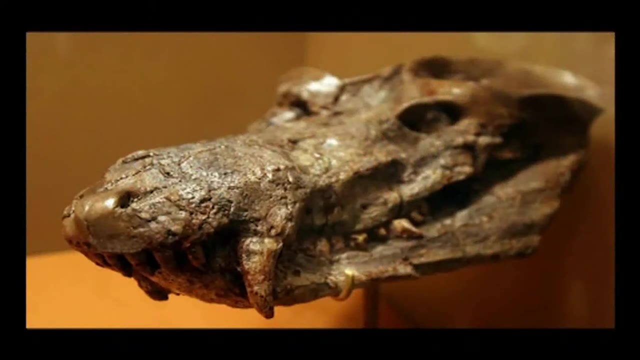 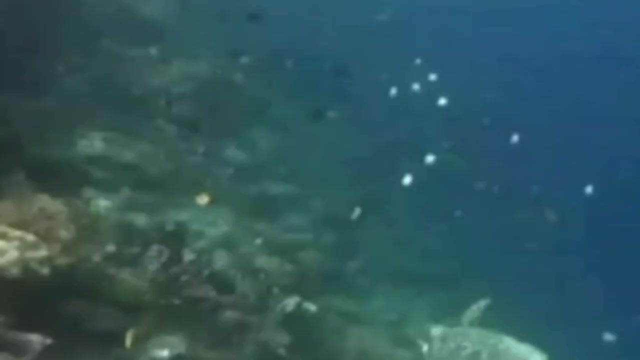 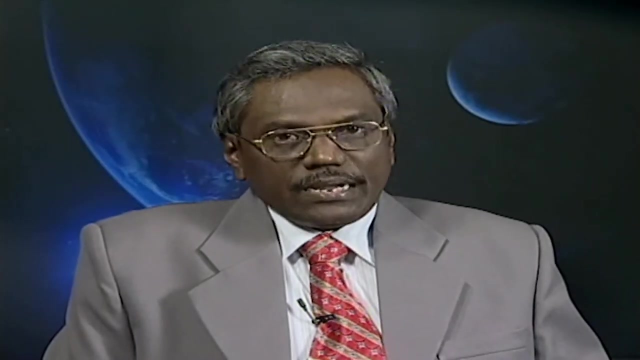 evidence: Land reptiles like Lystrosaurus, fossils from the rocks of same age from locations of South America, Africa and Antarctica are another evidences. Several living animals are being found on different continents even today. The widespread distribution of perma-carboniferous sediments in South America, Africa, Madagascar. 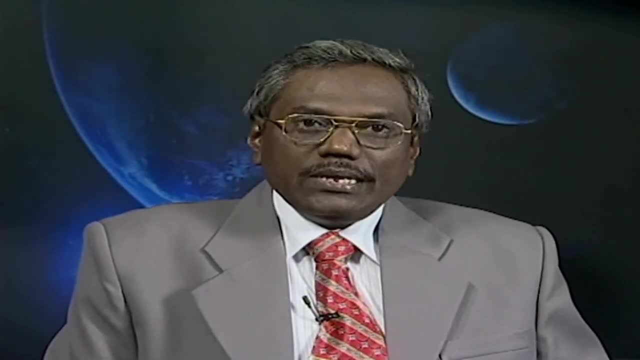 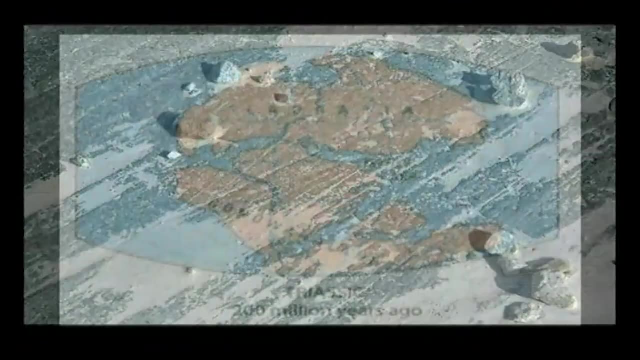 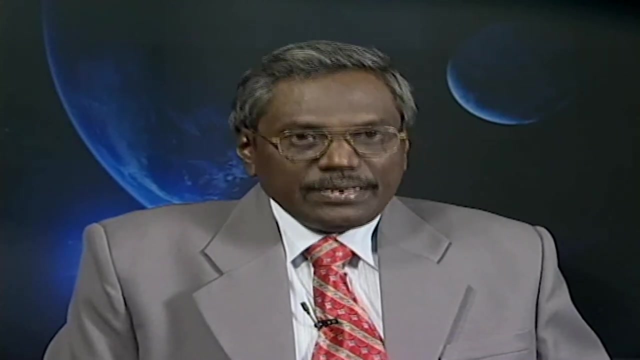 Arabia, India, Antarctica and Australia is another evidence. The oriented glacial striations and deposits called as stillites in the Gondwana land was another evidence. Similar coal deposits existing in the eastern United States and Siberia is one more evidence to support the theory of continental drift. 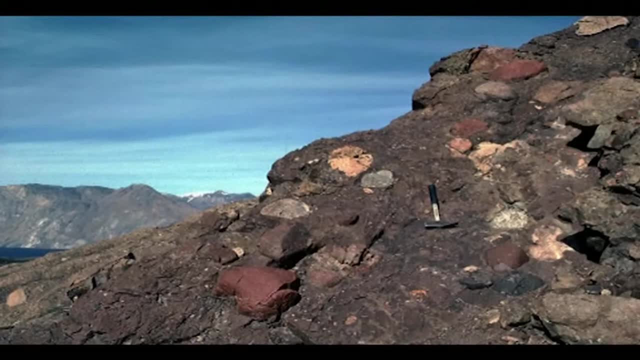 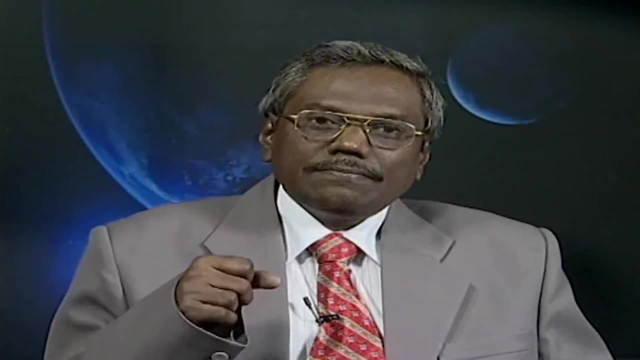 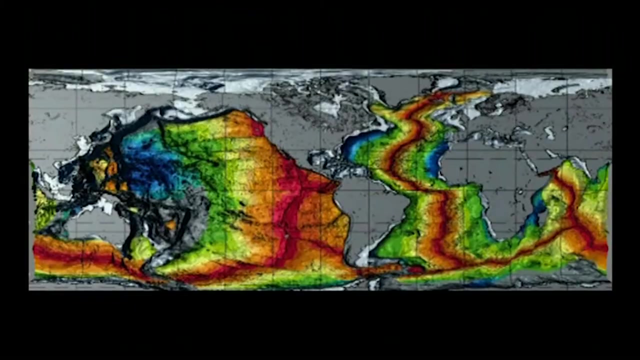 Rocks of different ages show a variable magnetic field directions- Magnetic north and south, reverse through time, which have been seen in different rock types. Initially it was considered as polar wandering and later it was attributed to palaeomagnetism and finally it has led to the theory of plate tectonics. People mistook the palaeomagnetism with reference to polar wandering. The study of palaeomagnetism is a theory of the entire geological groups. The study of palaeomagnetism is a theory of the entire geological groups. The study of palaeomagnetism is a theory of the entire geological groups. 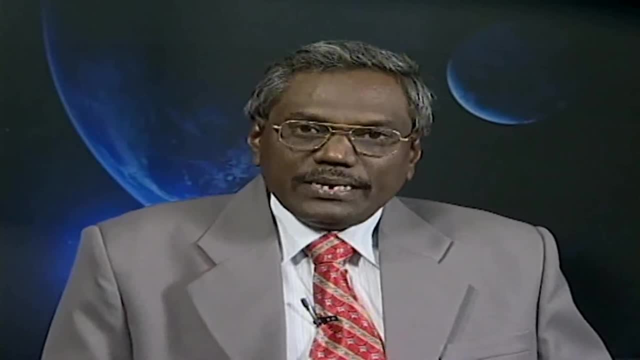 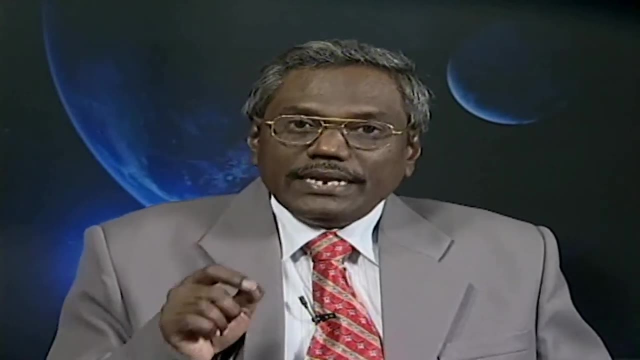 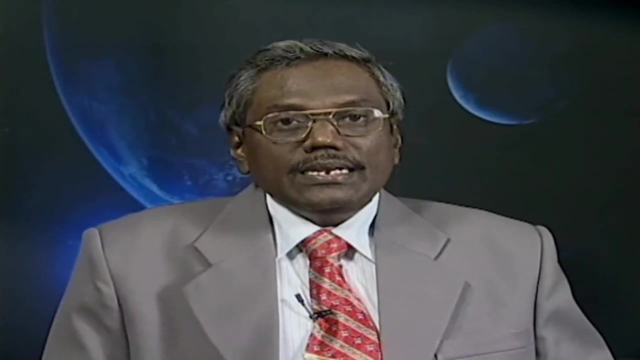 came after these studies. This has provided the geophysical evidences to support the movement of lithospheric plates. The word plate here technically refers to the rock mass which is available on the crest Early in 1953. scholars have introduced the theory of plate tectonics. 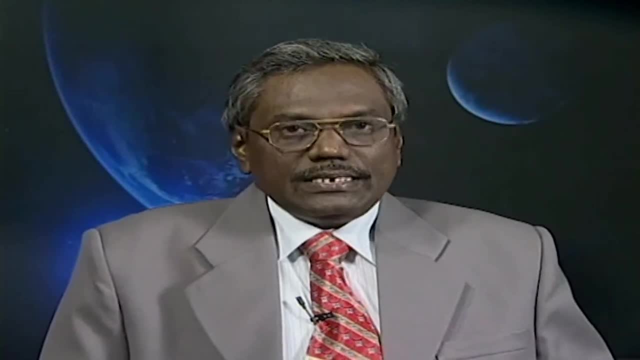 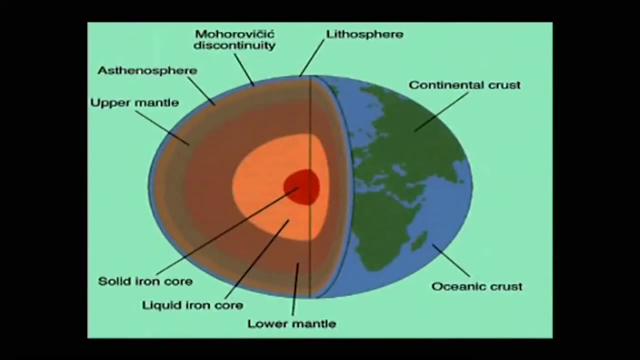 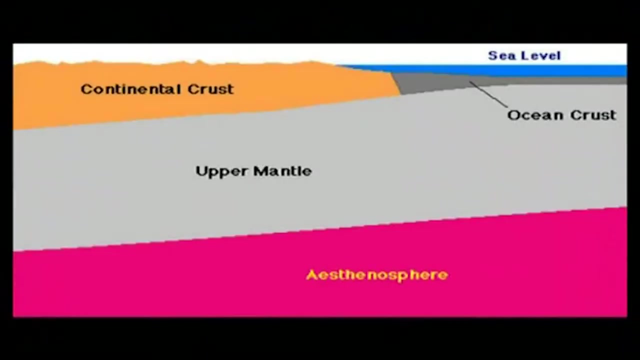 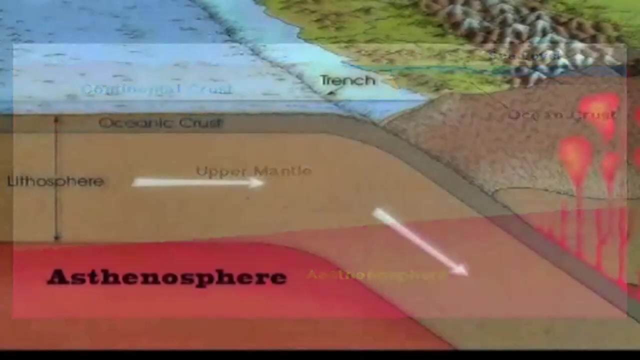 Jack Oliver, a geophysicist, provided many seismological evidences for these findings. Continental crest, oceanic crest and lithospheric plates were identified as unique features. after this, Scientists believe that below the lithosphere there is a relatively narrow mobile zone in the mantle called as asthenosphere. 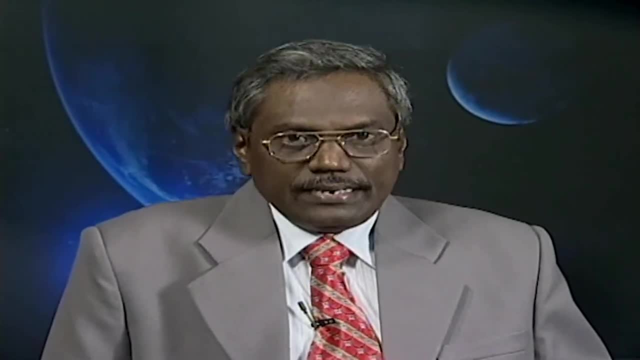 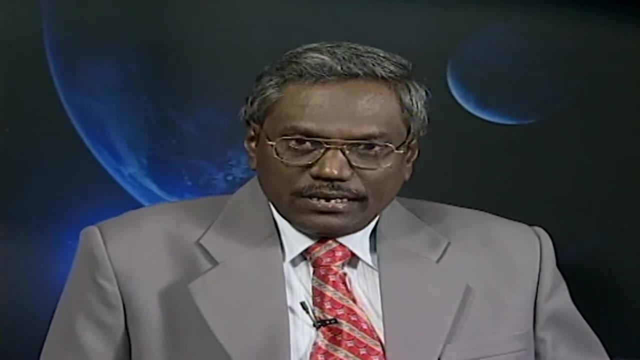 This zone is composed of three components. The first component is the geophysical plate and the second component is the geophysical plate. The geophysical plate is the geophysical plate which is composed of hot, semi-solid material which can soften and flow after being subjected to high temperature and pressure over a geological time. This rigid lithosphere 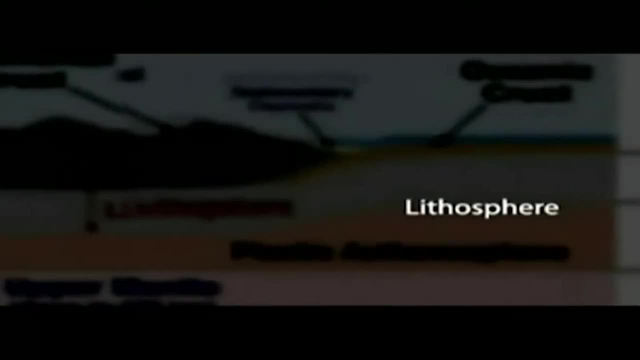 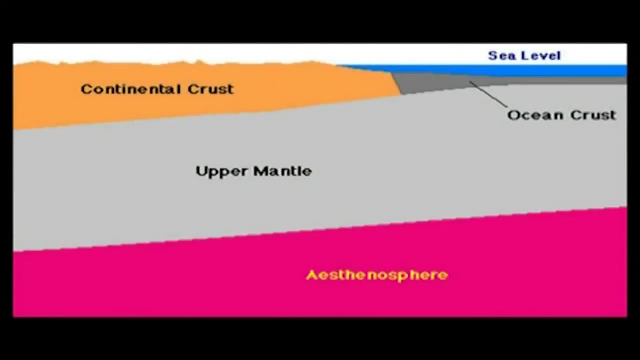 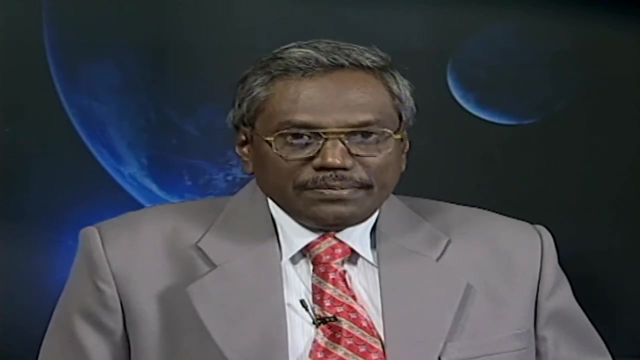 is thought to float or move on the slowly flowing asthenosphere. This diagram shows the position of asthenosphere in the interior of earth. It illustrates the location of asthenosphere approximately 100 kilometers below the surface and 60 kilometers below the continental and. 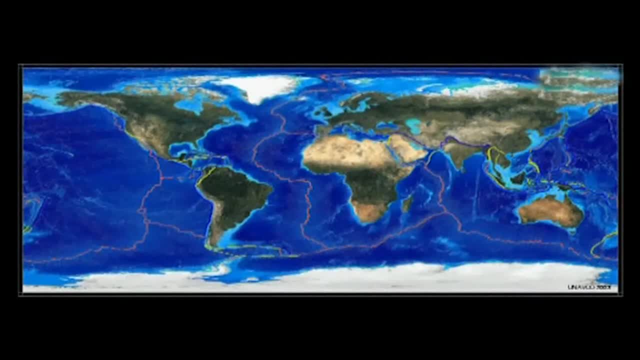 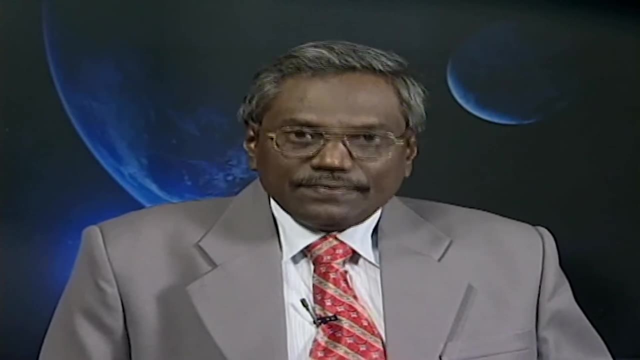 oceanic crest. Lithosphere is broken up into seven to eight major tectonic plates and several minor plates. These plates are viscoelastic solid rock bodies. A tectonic plate is a massive, irregularly shaped slab of solid rock. The plate is a imposed on the surface and the surface of 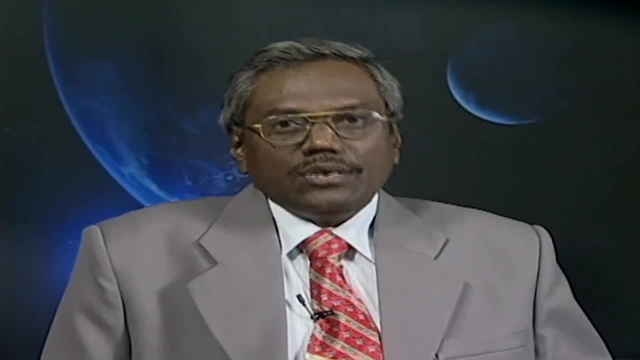 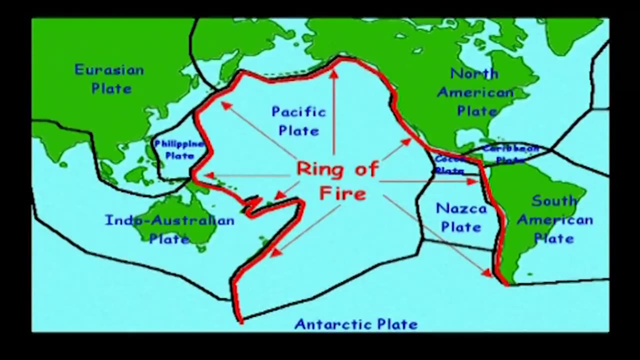 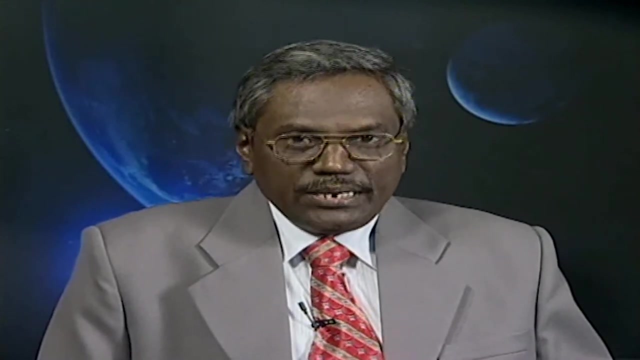 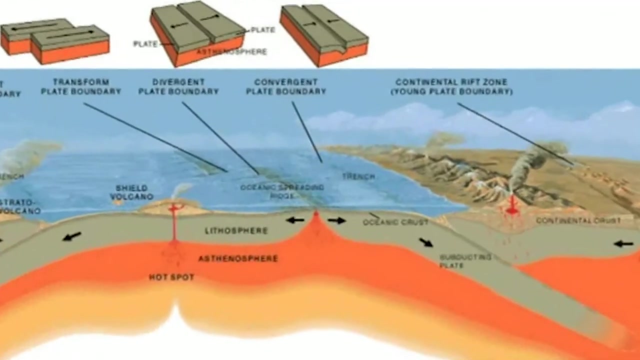 The plate size can vary greatly, from a few hundred to thousands of kilometers across The Pacific and Antarctic. plates are among the largest plates. Plate thickness also varies greatly, ranging from less than 15 kilometers for young oceanic lithosphere to about 200 kilometers or more for ancient continental lithosphere. 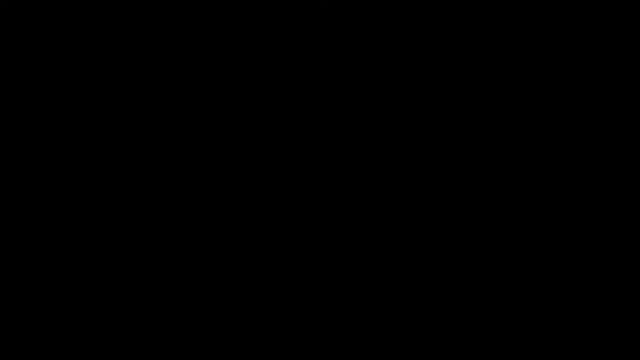 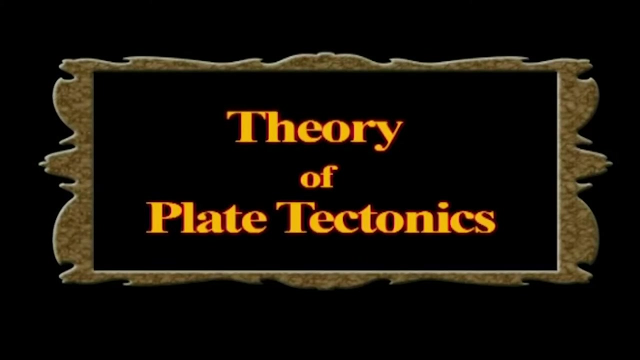 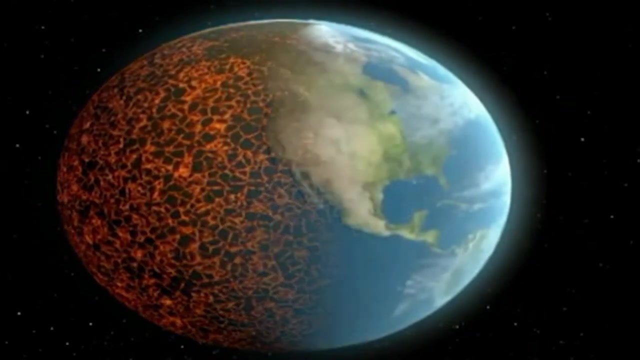 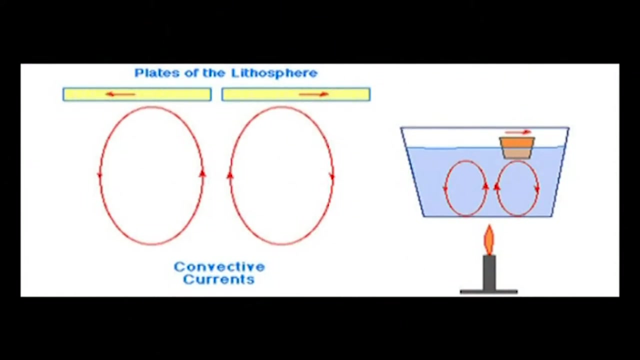 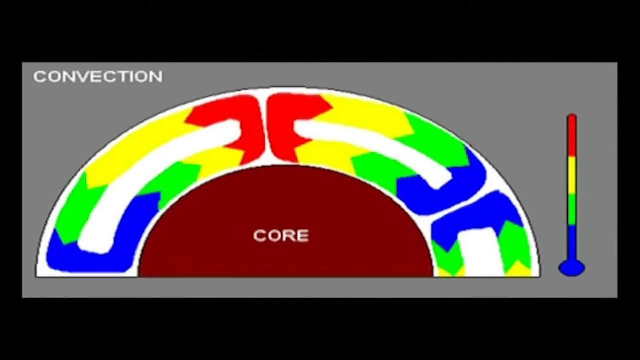 Plates ride on the asthenosphere. The radiation from the earth's interior generates convection currents, which move the plates apart. This diagram shows illustrates the movement of plates due to convective currents. The convective currents move the plates apart, So there will be side waves. 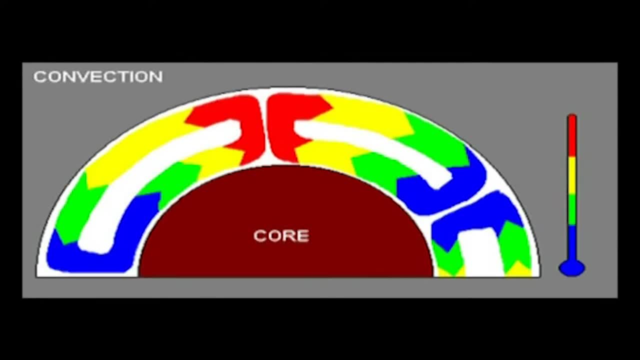 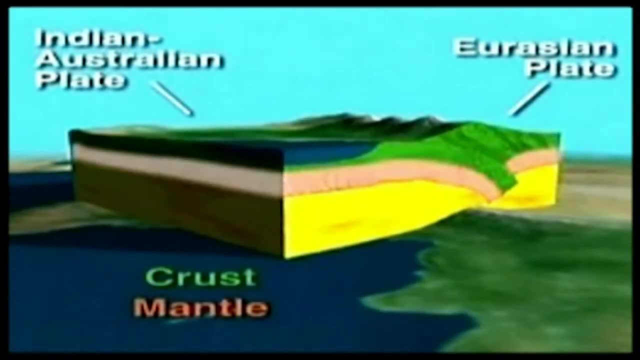 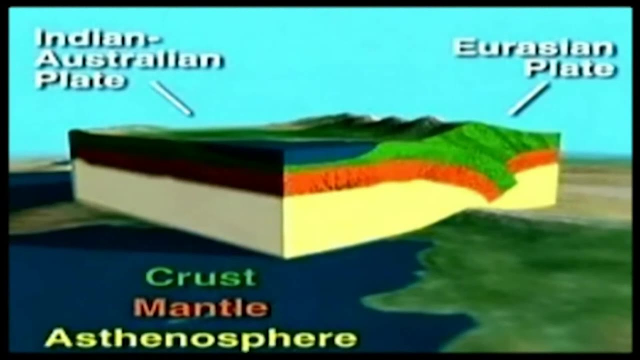 There will be inward movement of plates when the heat rises up towards the crest. The theory of plate tectonics describes the large scale motions of earth's lithospheric plates. Plates move in relation to one another. The location where two plates meet is called as plate boundaries. 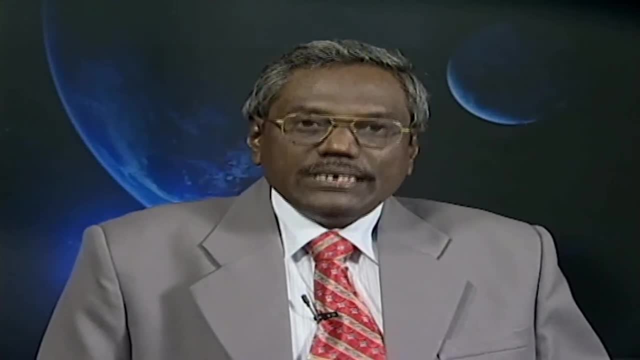 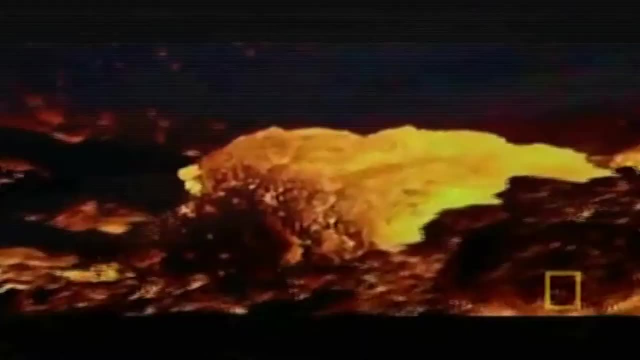 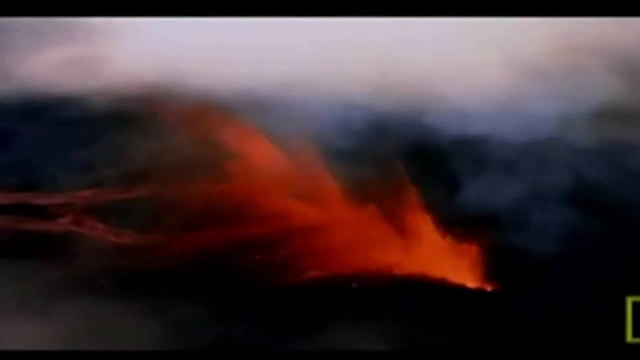 These areas are commonly associated with geological events such as earthquakes and the creation of topographic features like mountains, volcanoes and oceanic trenches. Plate boundaries are the home of the majority of the world's active volcanoes, with the Pacific plate's ring of fire. Plate movements happen along three types of plate boundaries, called as convergent boundaries, divergent boundaries and conservative transform boundaries. Let us see the earth's crest and asthenosphere, where two plates collide each other and where two plates move apart from each other and diverging plate goes into the earth, creating 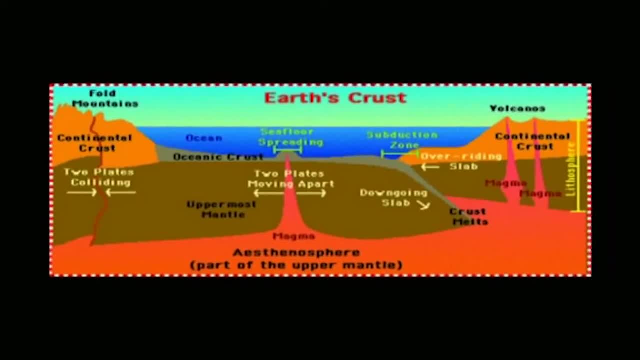 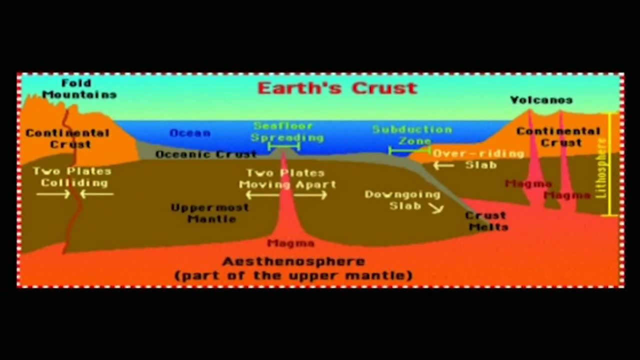 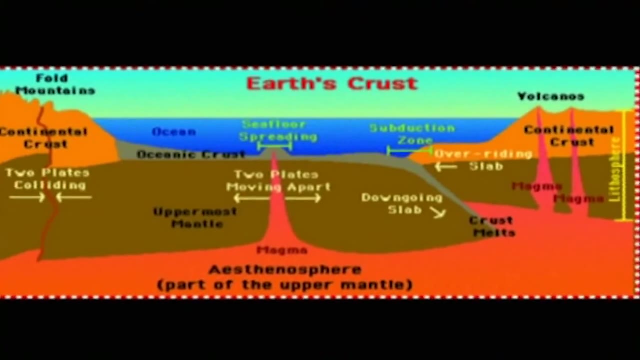 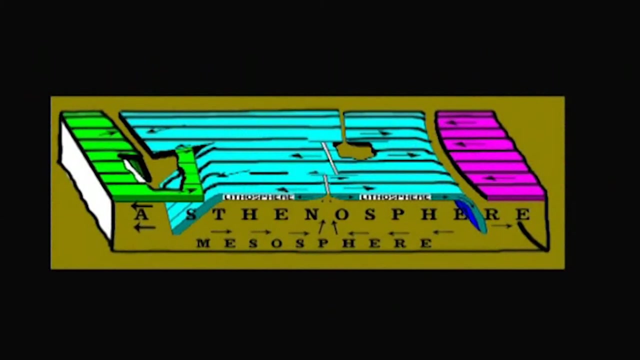 a lot of structures above the surface. At one particular area, you can see two plates are colliding each other at the continental crest, forming the fold mountains. In the middle of the diagram, we are seeing two plates moving apart from each other, creating the spreading of sea floor. In the right hand side of this diagram, we are seeing a diverging 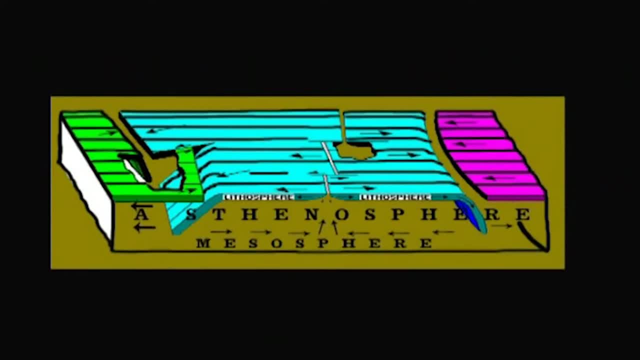 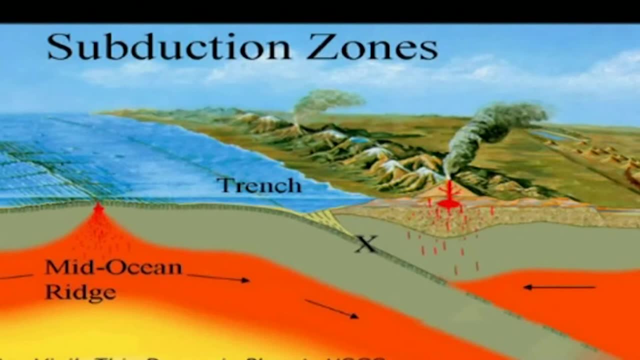 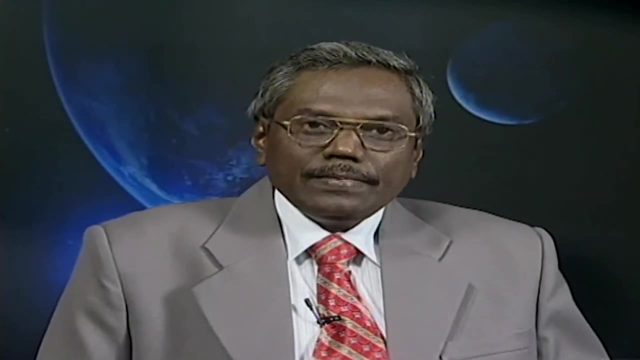 plate which is going inside the crest, creating a rift along the boundary wherein the zone goes into the interior, called subduction zone. So three types of impacts can be expected during this process: The fold, mountains are raised up, sea floor gets spread up and the 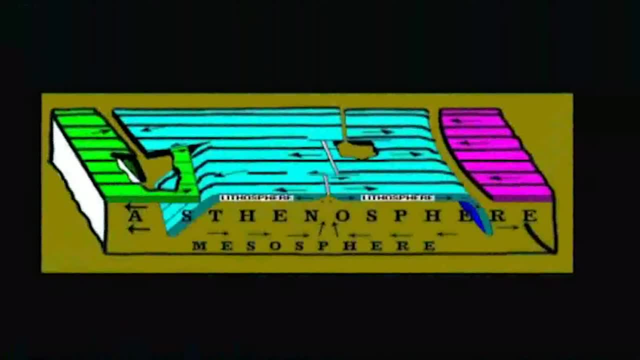 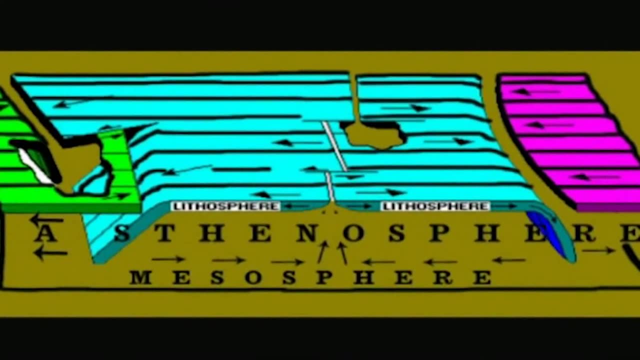 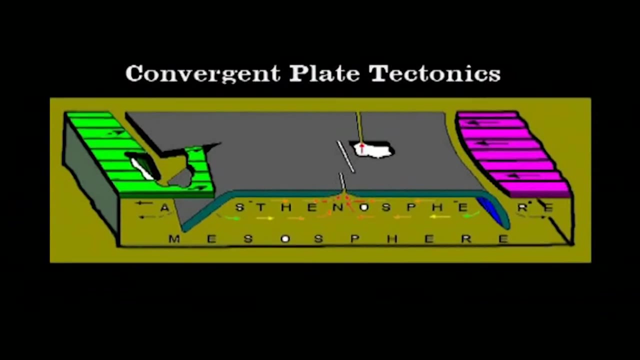 oceanic zone goes in as subduction zone. The divergent plate tectonics model is shown in this diagram, wherein the plates move apart from each other, which may create a sea floor spreading. The convergent plate tectonics model is shown in this diagram, wherein the plates move towards. 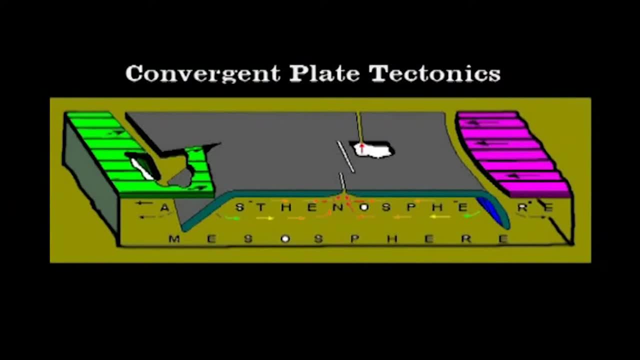 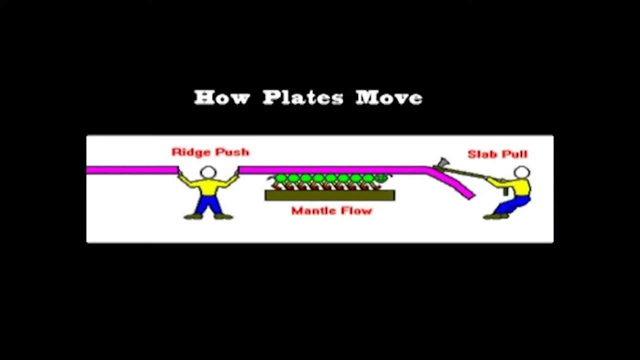 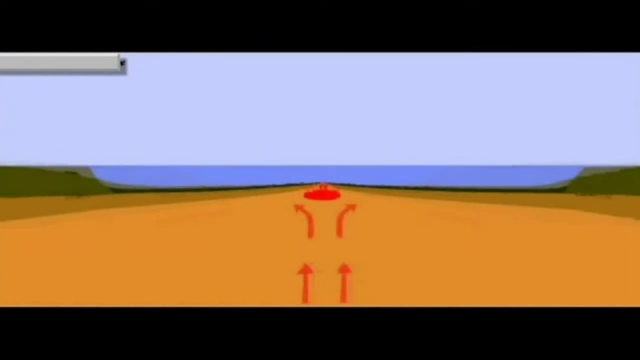 each other. Therein, mountain building processes, orogenic activities happen. This diagram illustrates how the plates move from one point to the other. Lateral relative movement of plates varies. It may range from 0 to 100 millimeter per year. Tectonic plates are thick over continental. 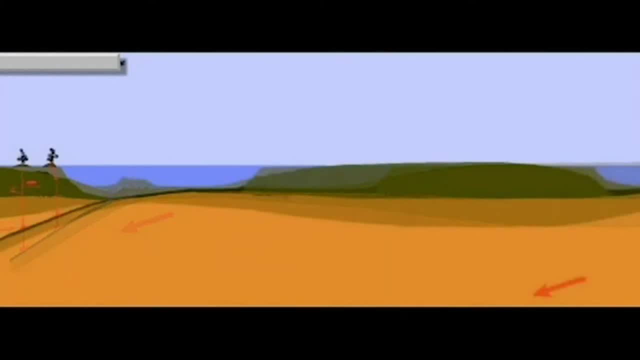 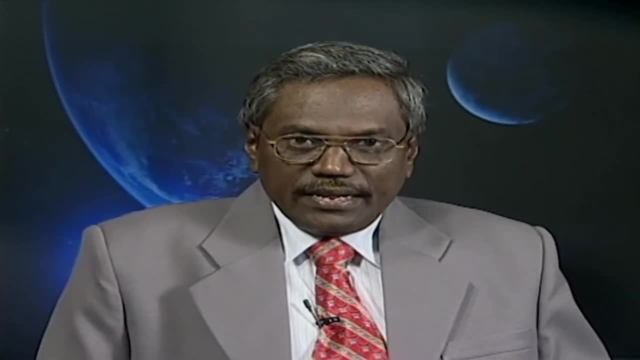 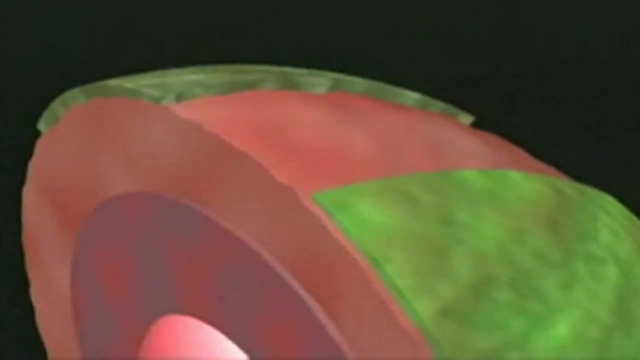 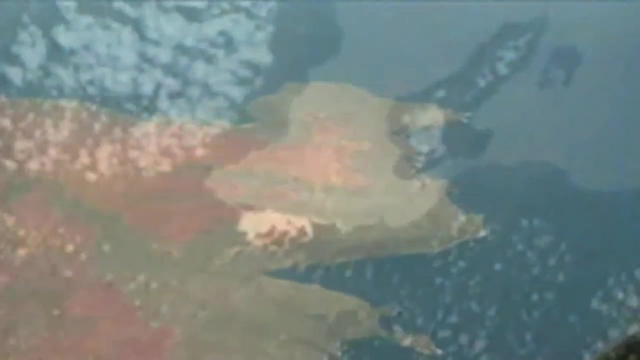 crest and thin over sea floor. Plates move because of the earth's lithosphere has a higher strength and lower density than the underlying asthenosphere Plate. tectonics is a kinematic phenomena. Dissipation of heat from the mantle is the source of energy for plate movements through convection. large 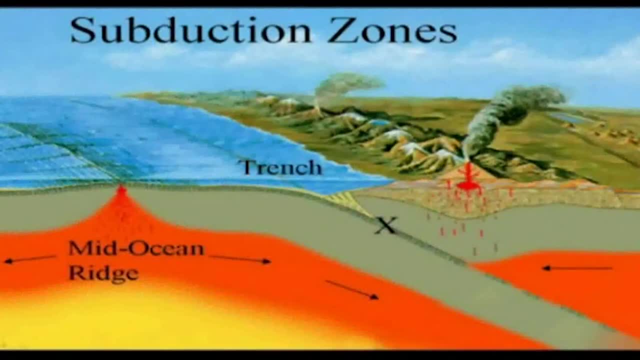 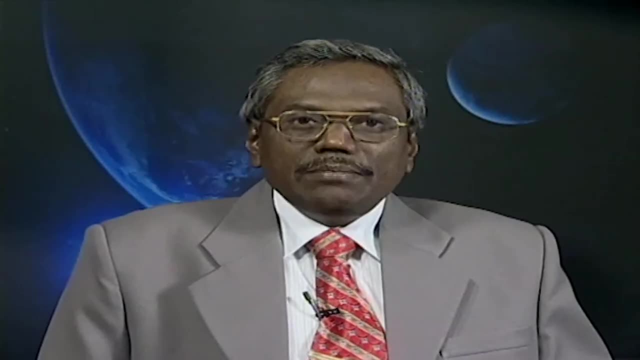 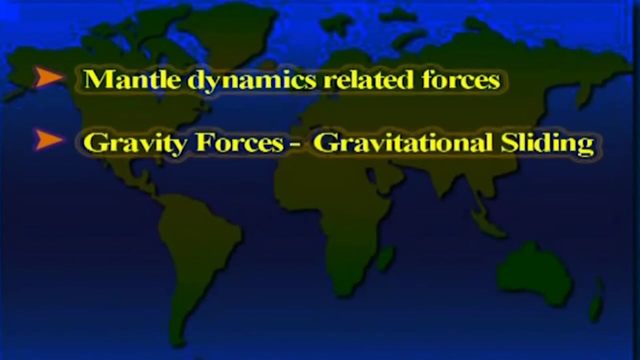 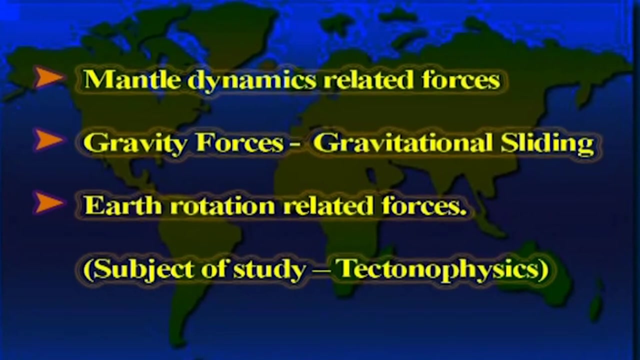 scale upwelling and doming. The weakness of the asthenosphere allowed the tectonic plate to move easily towards a subduction zone. Three major categories of driving forces exists in this: Mantle dynamics related forces, gravity forces or gravitational sliding earth rotation related forces, which all come under the subject. 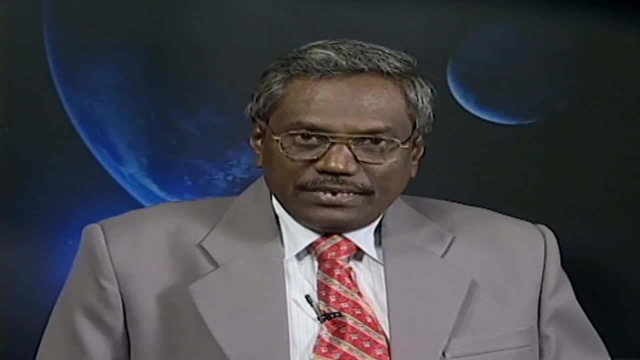 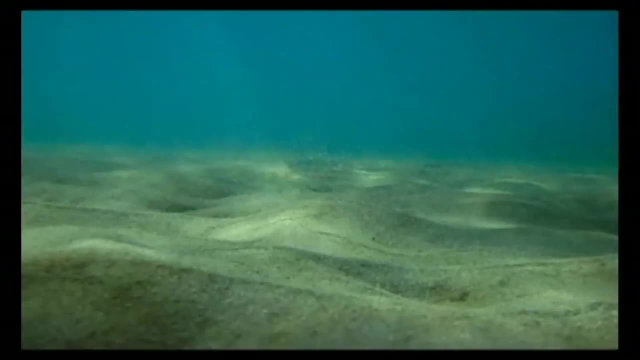 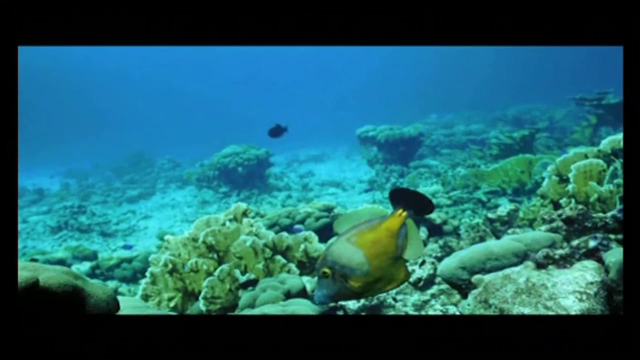 called tectonophysics. The Worls bathymetric observations of 1947 have shown the mid oceanic ridge of the central. The floor of the seabed beneath the layer of sediments consisted of basalt and not granite. Oceanic crust was much thinner than continental crust. 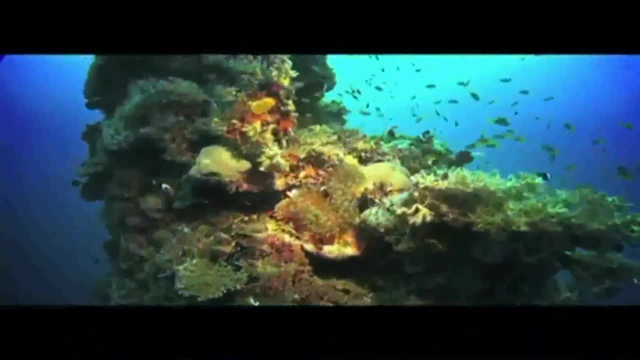 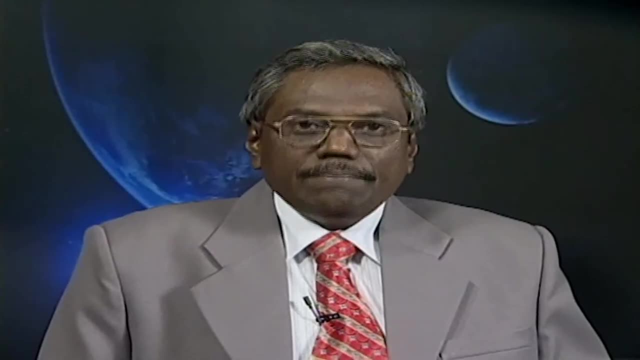 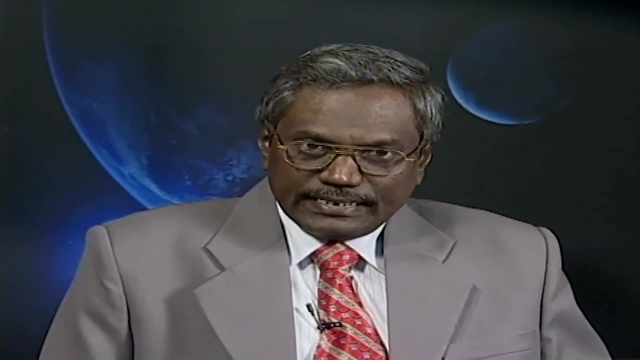 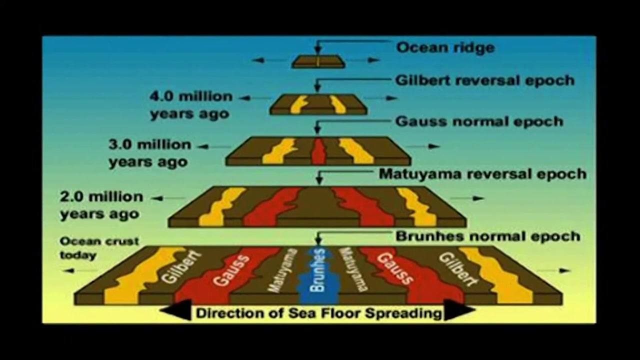 It was identified that the sea floor is spreading In 1950, detailed underwater explorations with geophysical instruments provided magnetic stripping along the mid-oceanic ridges. The sea floor spreading hypothesis was proposed in the year 1966.. This diagram illustrates the direction of sea floor spreading at different stages. 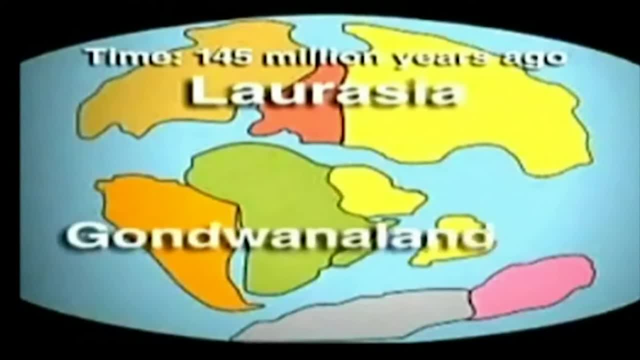 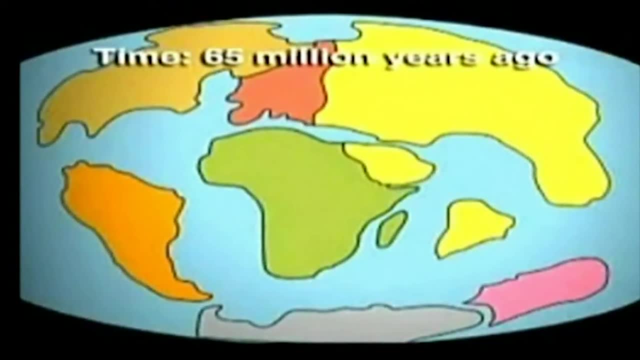 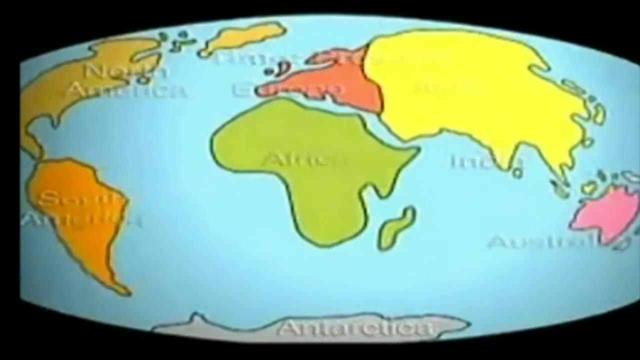 Pangaea started to break up into two smaller super continents called Laurasia and Gondwana land during the late Triassic. By the end of the Cretaceous period, the continents were separating into land masses that look like our modern day continents. 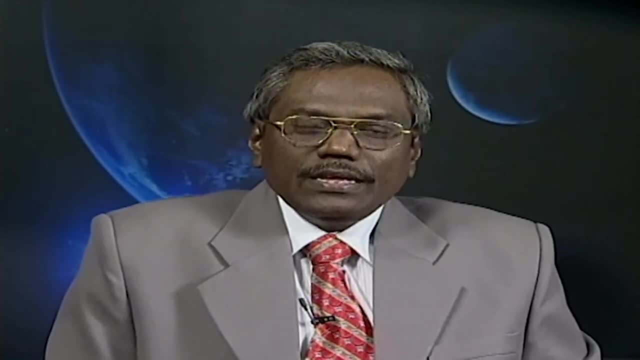 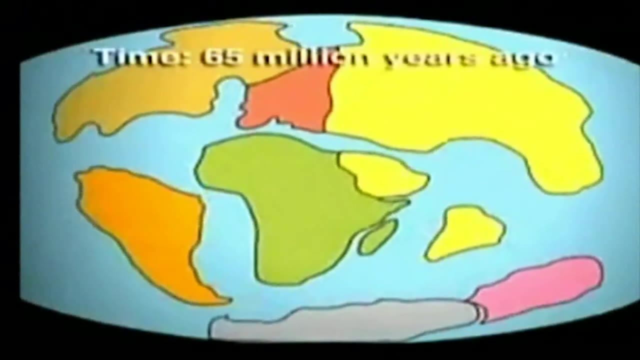 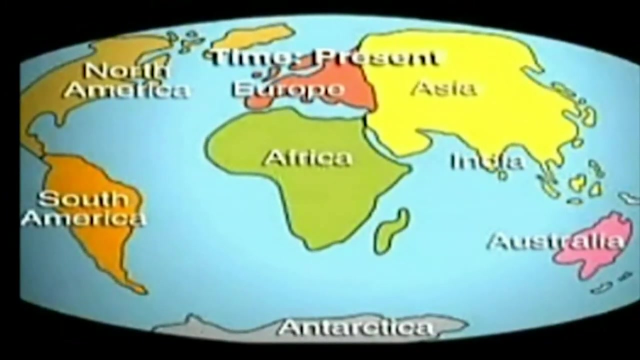 It formed the continents Gondwana land and Laurasia, which got separated by the Tethys sea. When the supercontinent Pangaea broke into Laurasia and Gondwana land, all the oceans got originated. So this is the point where the origin of ocean happened. 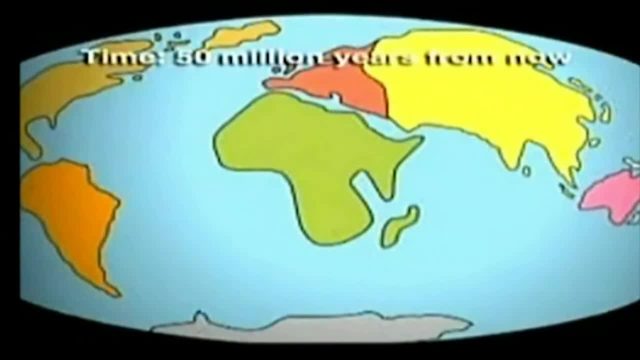 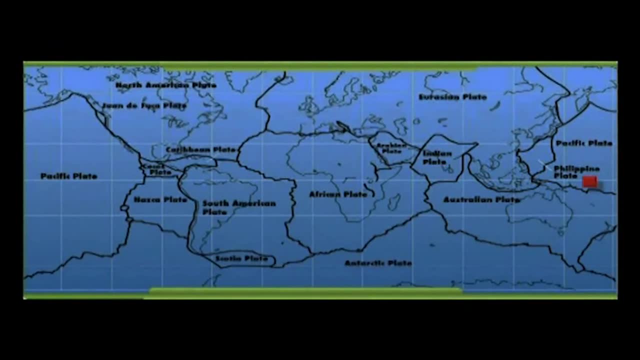 The current continental and oceanic plates which are in existence are the Eurasian plate, Australian Indian plate, Philippine plate, Pacific plate, Juan de Fuca plate, Nazca plate, Caucasus plate, North American plate, Caribbean plate, South American plate, African plate, Arabian plate, the Antarctic plate and the. 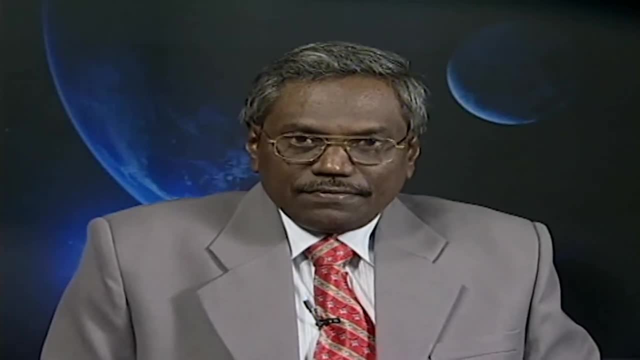 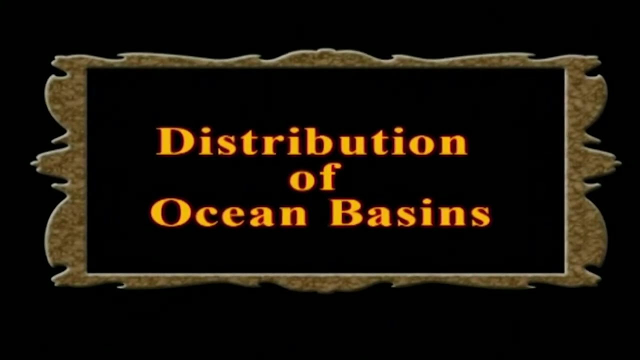 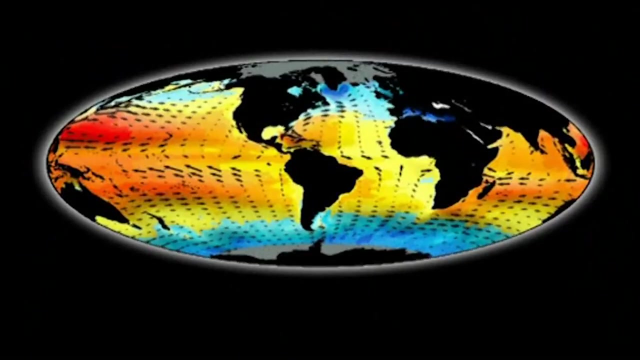 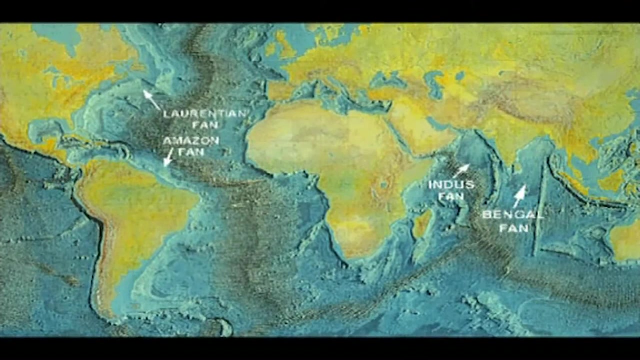 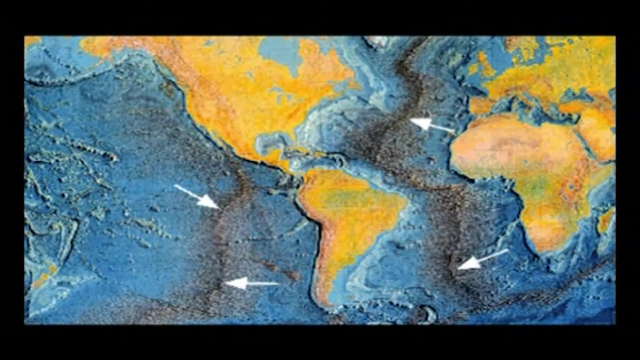 Scotia plate. These plates consist of smaller sub-plates. also, Let us see the distribution of ocean basins. Continents naturally divided the worlds. ocean basins, Continents and ocean basins are the fundamental relief features of the globe. They are considered to be the relief features of first order. 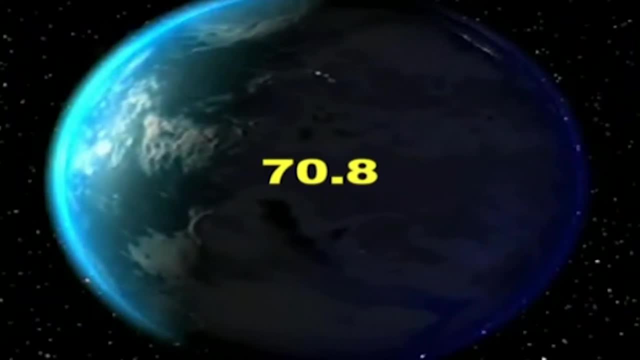 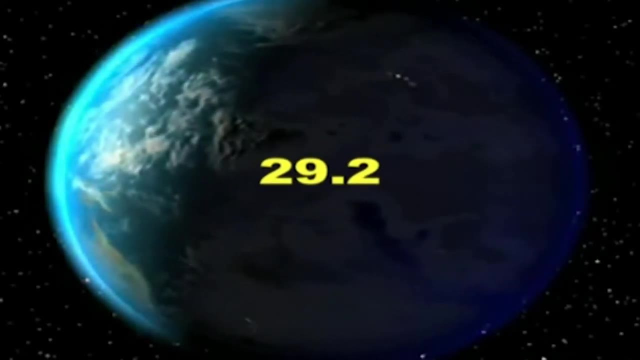 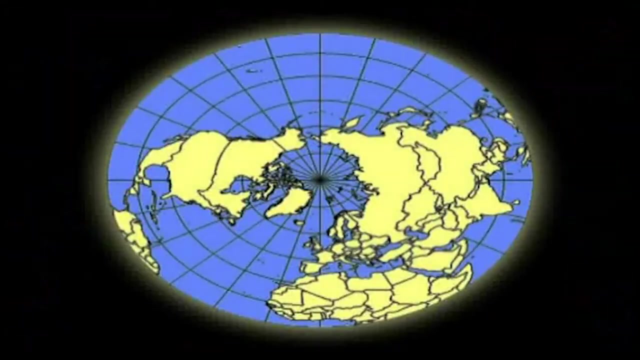 Today, about 70.8 percent of the total surface of the globe is represented by oceans and 29.2 percent is the surface is represented by continents. Let us see the distribution of oceans in the two hemispheres. In the northern hemisphere we have a different situation and in the southern hemisphere we 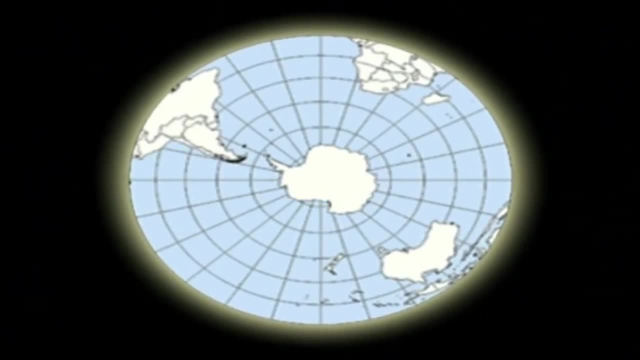 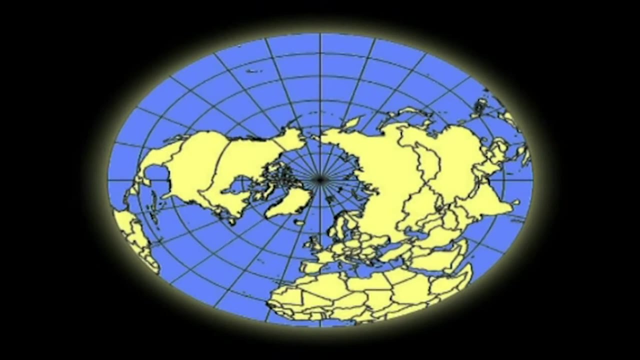 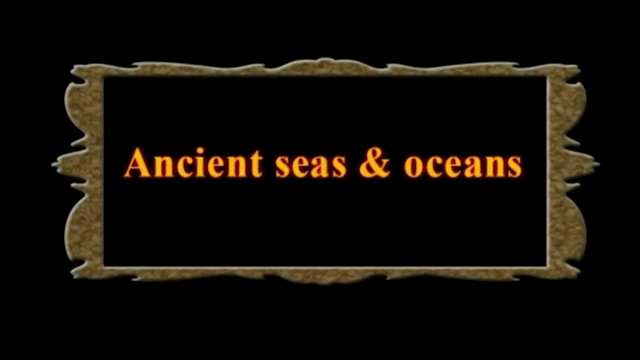 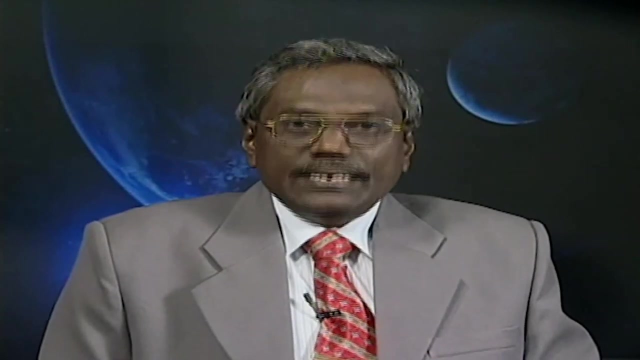 have got a different situation. We have overwhelming dominance of land areas in the northern hemisphere. More than 75 percent of the total land area is situated north of the equator. Hence the northern hemisphere is called as land hemisphere. Let us see the ancient seas and oceans. Roughly about 200 million years ago, there were only 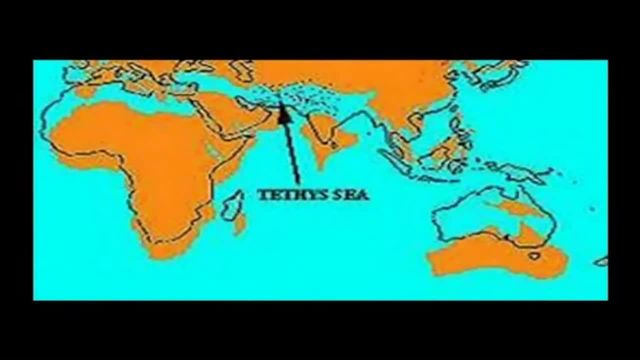 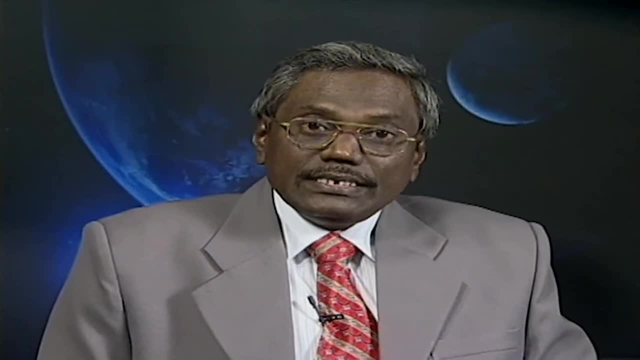 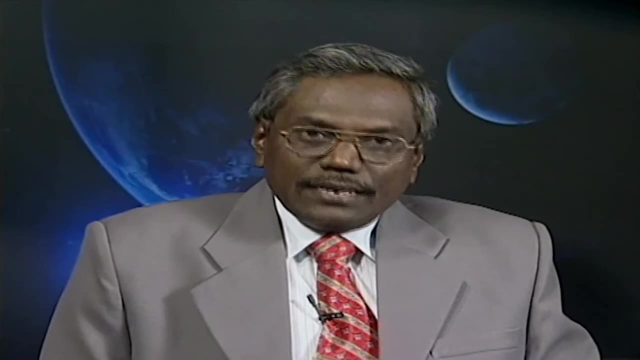 two water masses called as Pantelosa and Tethys Sea. Proto ocean surrounding the land mass. Pangaea was called as Pantelosa. This is the mother of all the oceans on earth. This was the primordial Pacific Ocean. Pantelosa word was derived from the Greek word meaning all sea. It was existing during 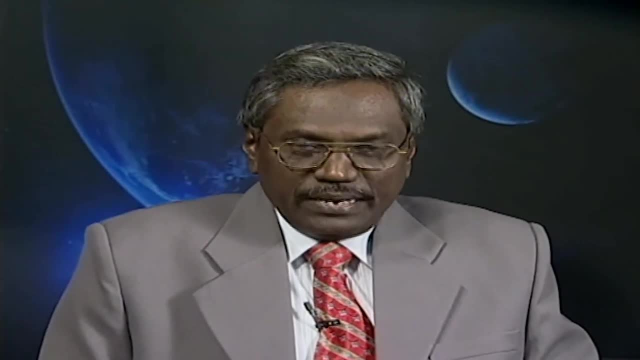 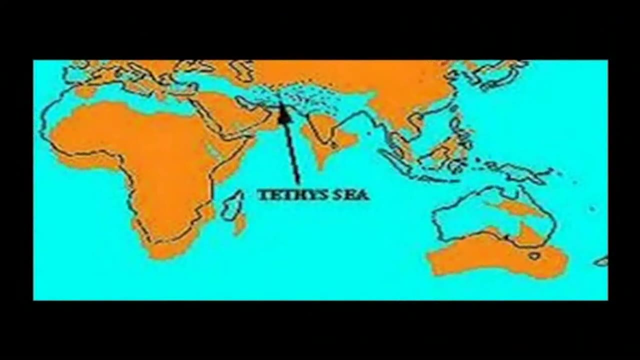 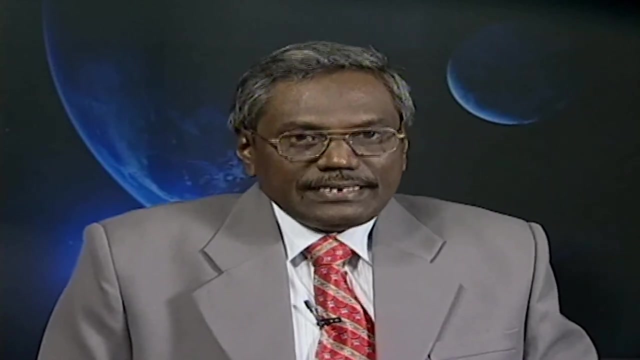 the late Paleozoic and the early Mesozoic period. It included the Pacific Ocean to the west and north and the Tethys Sea, or ocean, to the south east. It became the Pacific Ocean following the closing of the Tethys basin and the break up of Pangaea, which created 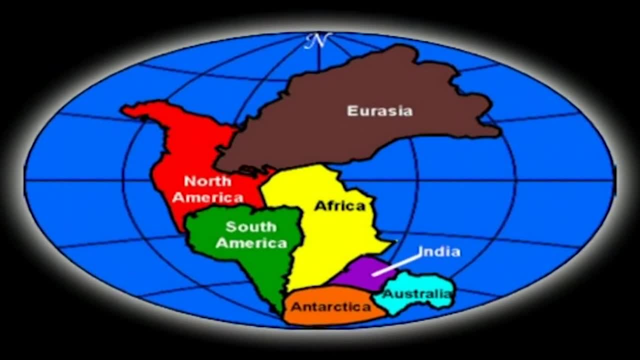 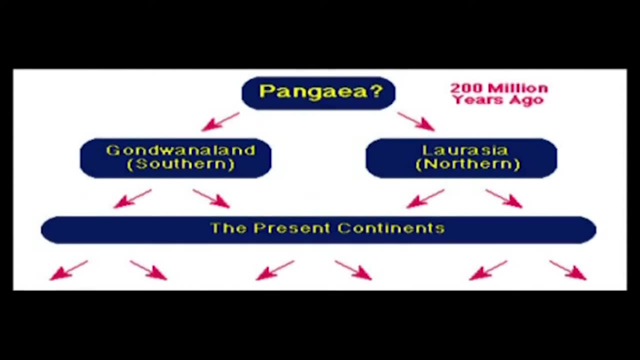 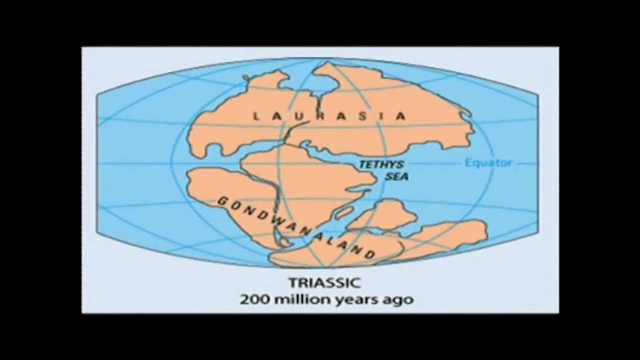 the Atlantic, Arctic and Indian Ocean basins. This diagram illustrates the break up of Pangaea into Gondwanaland and also Laurasia roughly about 200 million years ago. During the Triassic period. roughly about 200 million years ago, you can see the presence of Tethys and the 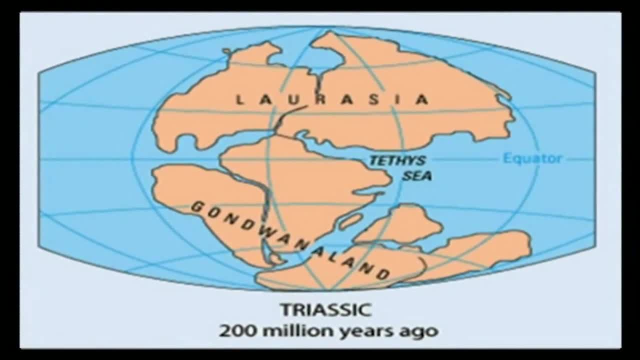 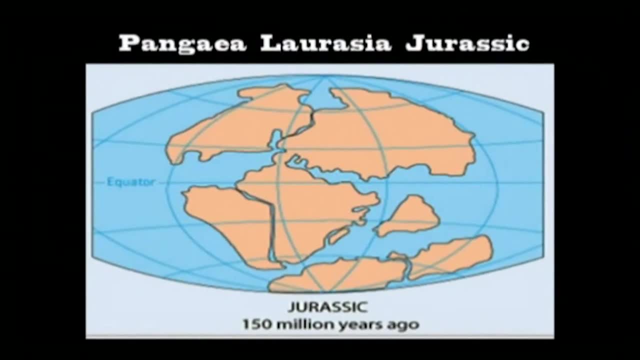 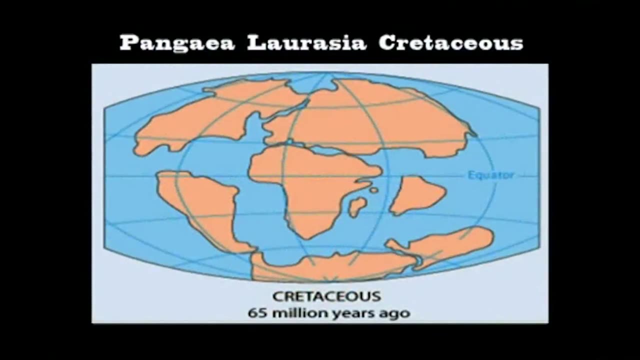 presence of the Tethys Sea. The Tethys Sea started to swing during this period. Roughly about 150 million years ago, during the period of Jurassic, the continents started moving away from each other. This diagram shows the position of the continents during Cretaceous. 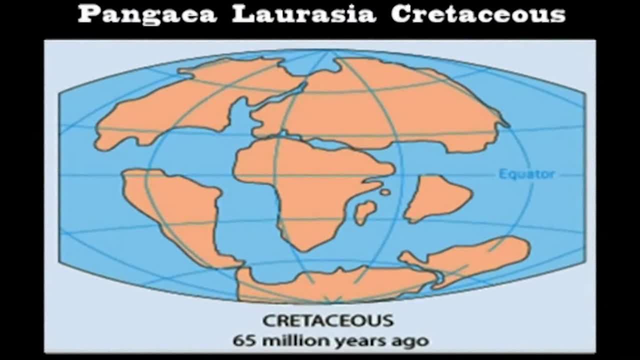 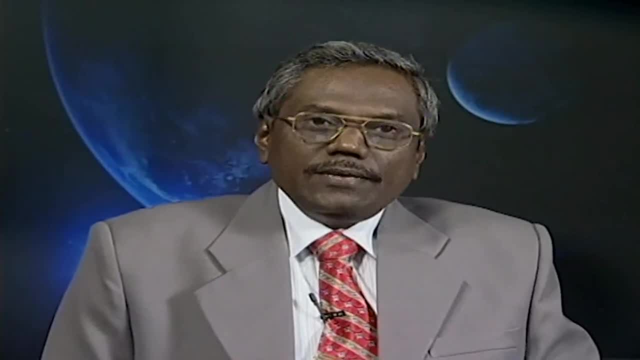 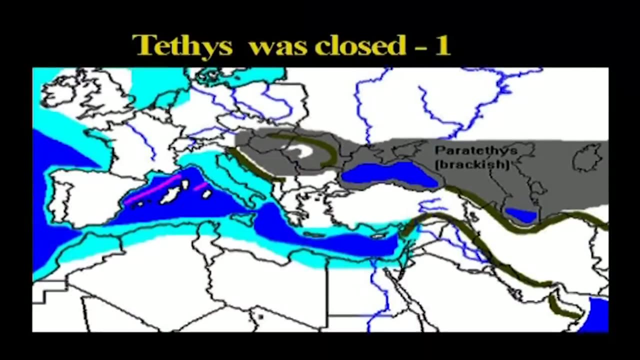 period roughly about 65 million years ago. This diagram shows the position of various continents and oceans today. Gradually, the Tethys Sea was closed and this diagram shows the stage 1 of the closure of Tethys Sea. It illustrates the Mediterranean region. 20 million years ago, The Tethys is. 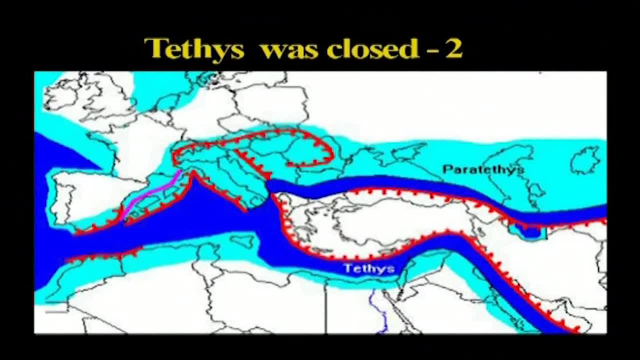 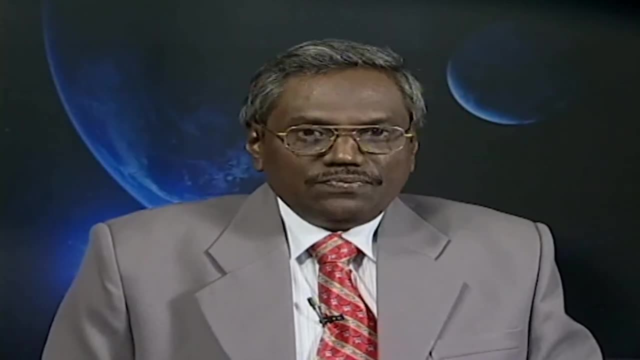 about to close as Africa and Eurasia converge each other. The stage 2 of the closure of Tethys Sea is shown here. By 10 million years ago, plate collisions have sealed off the eastern Mediterranean, trapping small remnants of ocean floor in the blackened Caspian seas. 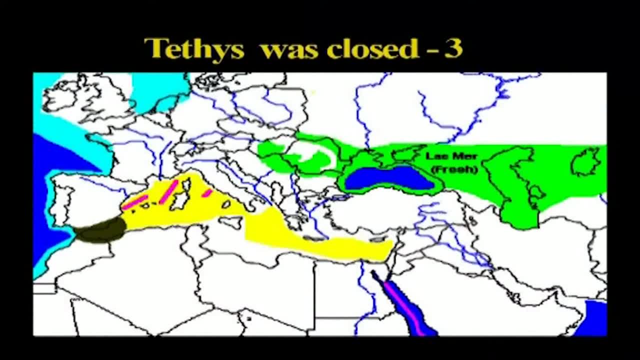 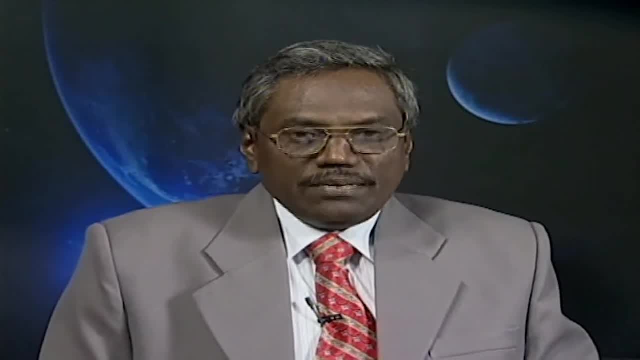 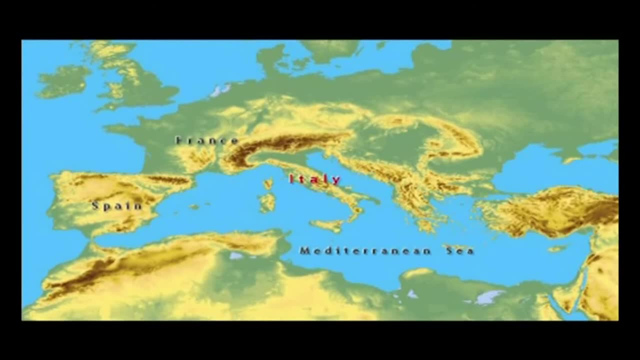 This diagram illustrates the closure of Tethys Sea at stage 3.. By 6 million years ago, Spain and Africa collide, raising a mountain barrier and sealing off the western end of the Mediterranean. The river inflow is not enough to maintain the level of the Mediterranean, which got 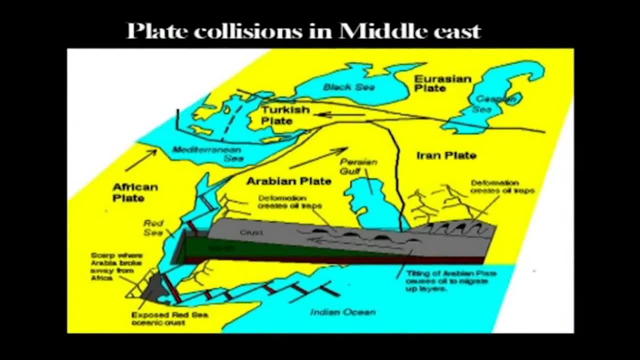 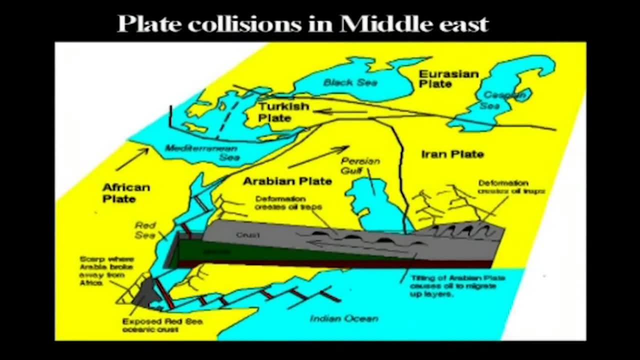 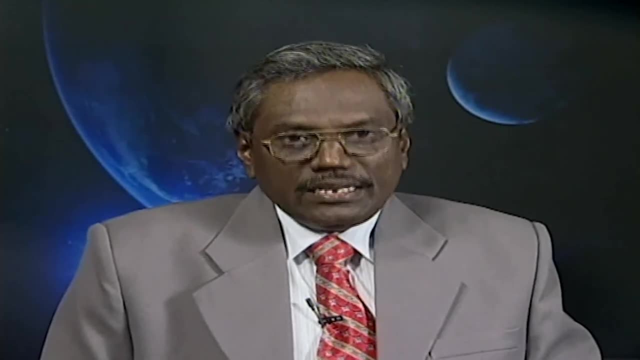 dried up. This diagram illustrates the plate collisions in the Middle East. The impacts are severe in the Middle East due to this plate collision. A lot of earthquakes, earth tremors and other activities happen. Mountain building processes also happen in the Middle East. India has fractured the crest of East Asia into several 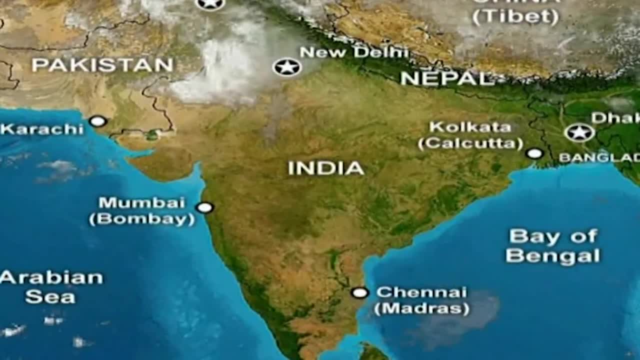 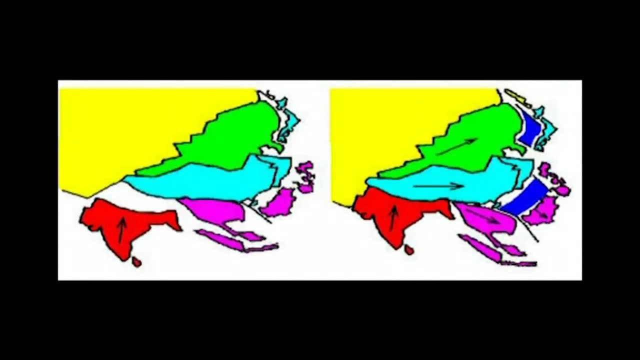 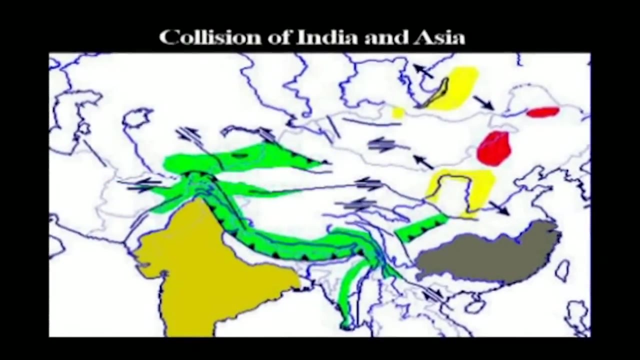 subplates which have been pushed far to the east and southeast as the collision has progressed. The diagram shows two stages of the movement of India towards North and North East, where the closure of Tethys Sea happened. The collision of India and Asia is shown in this diagram where, in the mountain building. 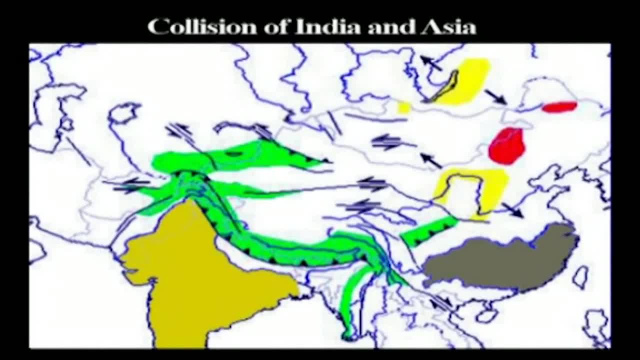 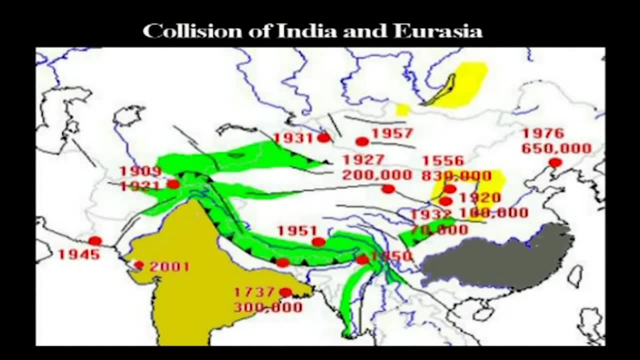 process happened where the Himalaya got rized up. The collision of India and Eurasia has created a lot of earth tremors and earthquakes during different periods of time, and all of them have been shown in this diagram with the values of death toll. 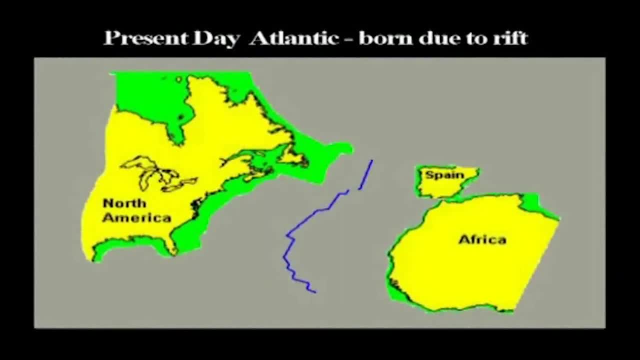 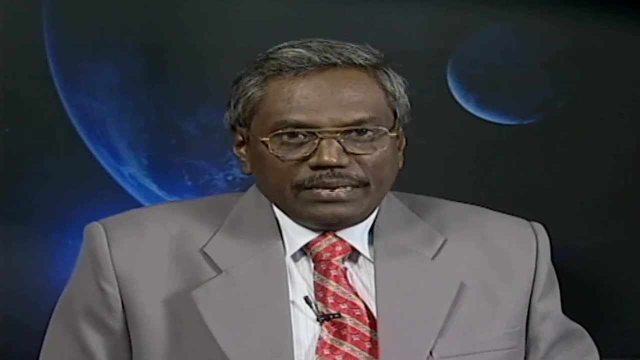 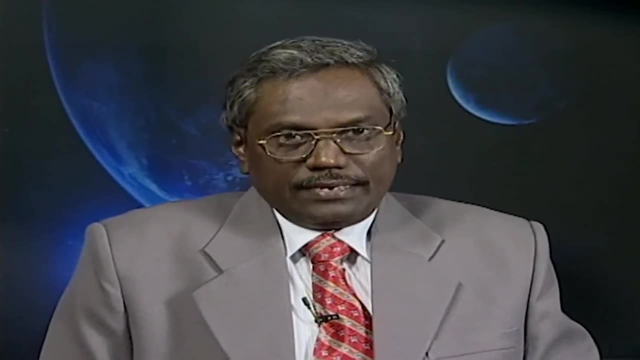 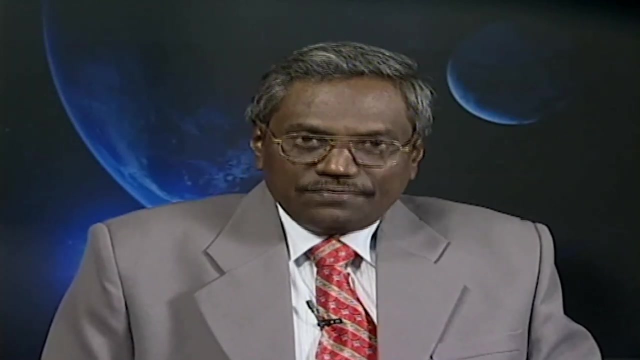 role. The present day Atlantic bond due to the rift is shown in this diagram. This diagram shows the Atlantic 65 million years ago. By 900 million years ago a triple junction formed as the supercontinent Rodinia started to rift apart. Between about 800 million years and 700 million years ago it split in half. 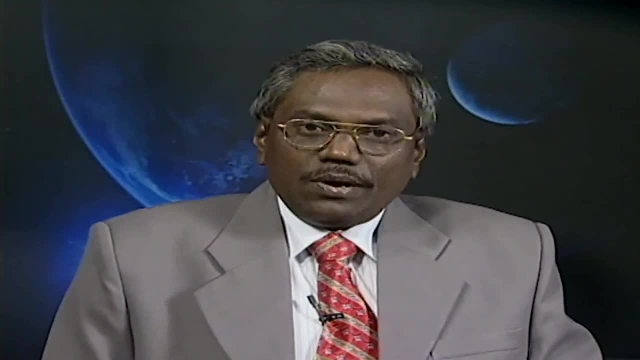 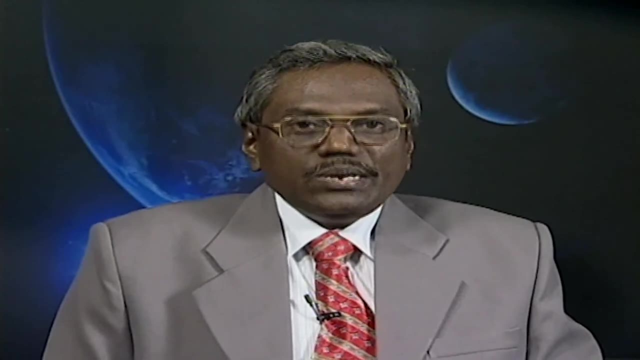 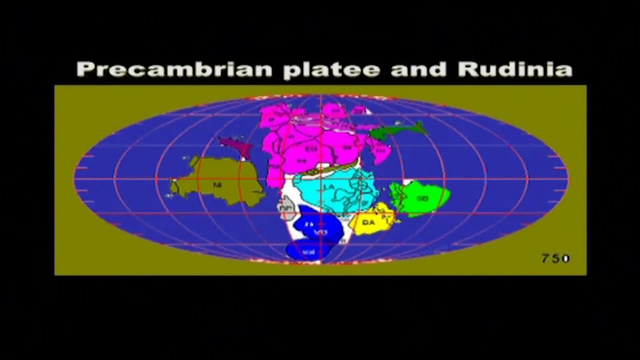 This was one of the most significant rifting events of all the times, because it opened up the panthelic ocean to the west of Laurasia and a continent that became North America. We are seeing the Rodinia and also the Precambrian plates, roughly about 750 million years ago. 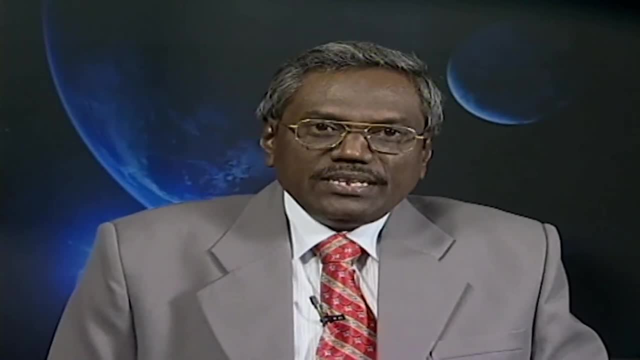 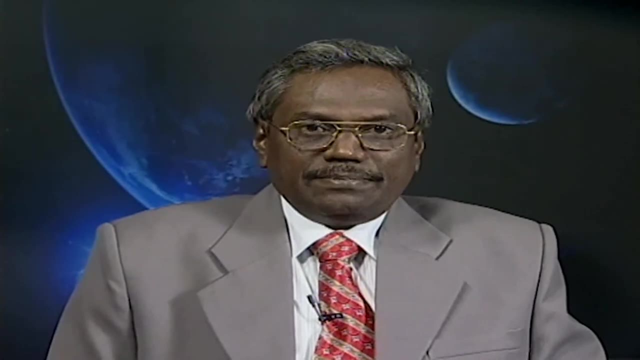 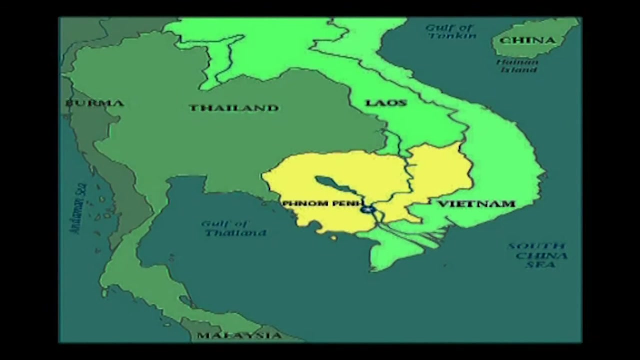 The global ocean of Mirovia, an ancient ocean that surrounded Rodinia, started to shrink because of the Pan-African ocean. The South China Sea opened as Borneo moved away from China. Also, Japan separated from the mainland, but it is not yet clear whether this was related. 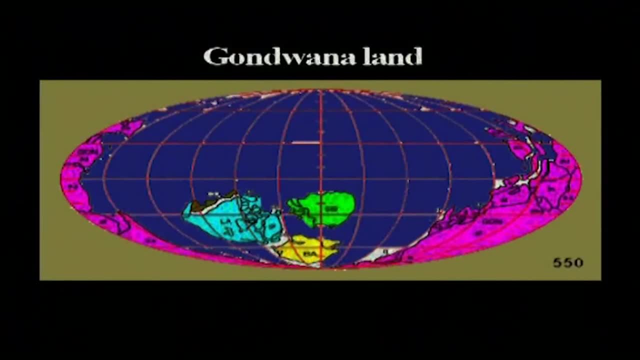 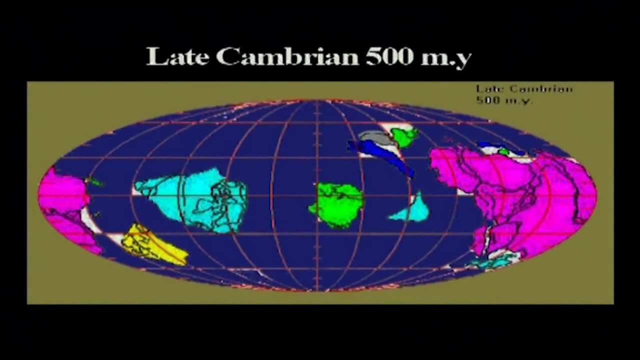 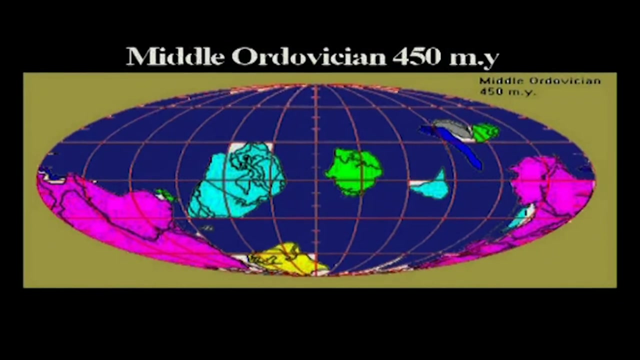 to the collision of India and Eurasia. This diagram shows the location of Gondwana land roughly about 550 million years ago. This diagram shows the position of the continents during late Cambrian period 500 million years ago. This diagram shows the middle Ordovician period world roughly about 450 million years ago.